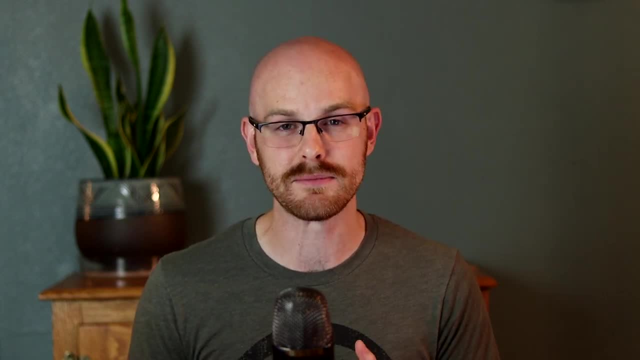 best to walk through everything, every single step of the way, and kind of explain all the concepts, And I'm going to talk a little bit about how to do that. So let's get started And so you can still learn something, even if you aren't super good at Python right now. With that, 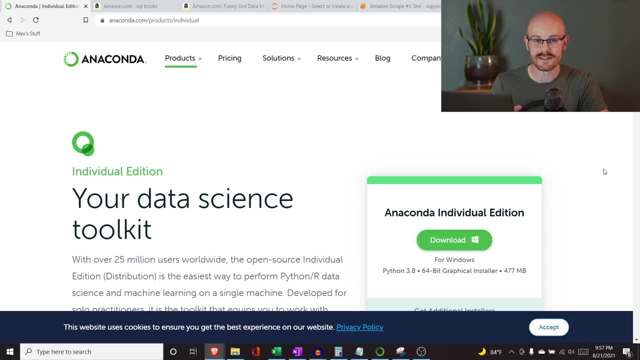 being said, let's jump over to my screen and get started on the project. All right, so we are going to get started, And if you didn't watch the last project, I had people download Anaconda. We use Jupyter Notebooks And I'll show you how to get to that in just a second, But I'll leave this link in. 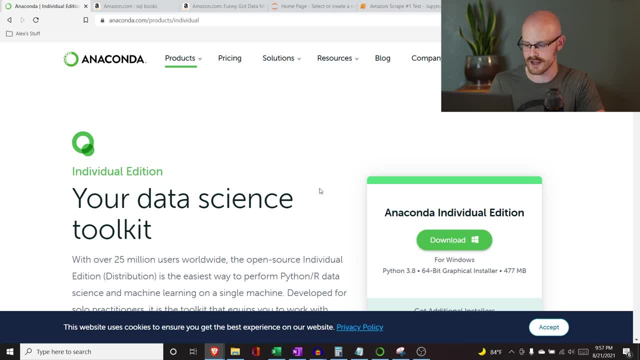 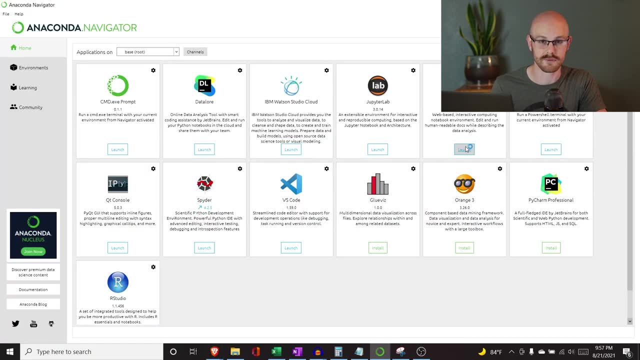 the description if you haven't done that already and you're just doing this project. But you'll go. you'll download Anaconda, you know, download super easy. And you're going to open up Jupyter Notebooks. I already have it open, But I'll open up another one just for you know the purposes of. 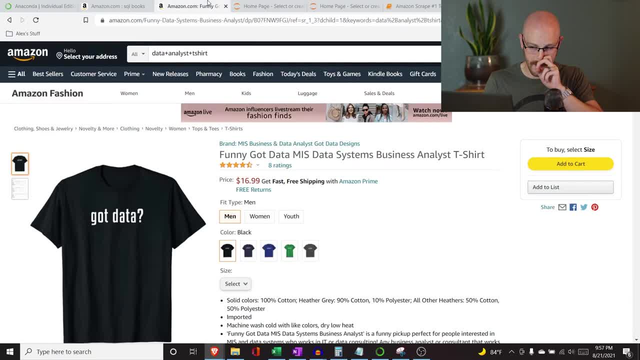 demonstration, What we are going to do today and what we, what people voted on. I mean, there's like there was like 8,000 people that voted in the poll that I made of what data you wanted me to scrape. There was like Amazon, cryptocurrency, weather, something else, I don't remember. 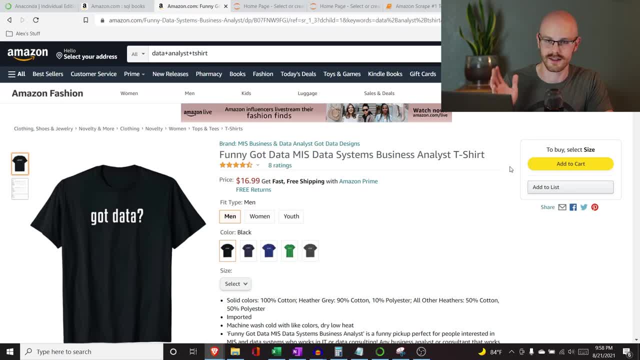 Overwhelmingly- I mean like 70% of people, maybe even 80%- Don't fact check me on that- Voted for Amazon, And so I'm going to do it Now. there are many things that you can scrape off of Amazon. 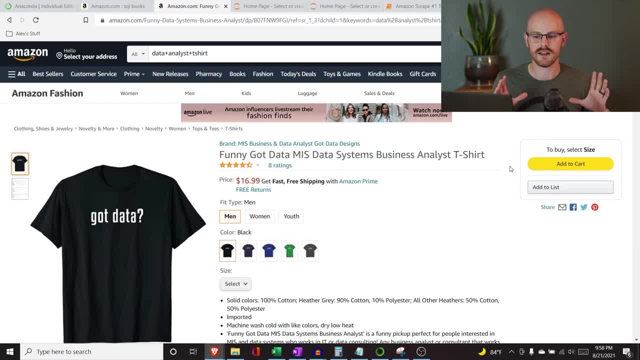 just a ton of stuff And I'm going to show you how to do it. I'm going to show you how to make it useful, how to make a data set, And it's going to be really interesting. But there are lots of. 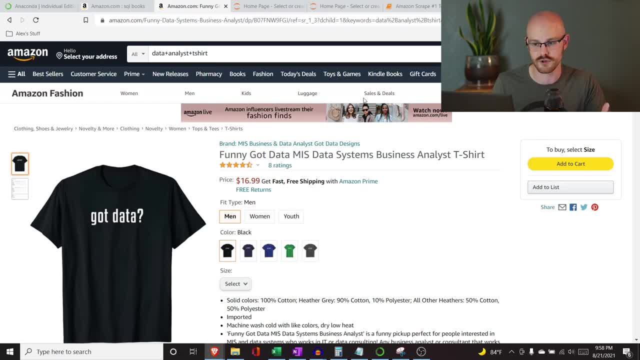 other ways to do this, And so I think- and I have already kind of created it- I'm going to show you an item and you can scrape, you know basically anything in here, And I'll show you how to do that. Another thing that is a little bit more advanced and that's why this first video is starting off. 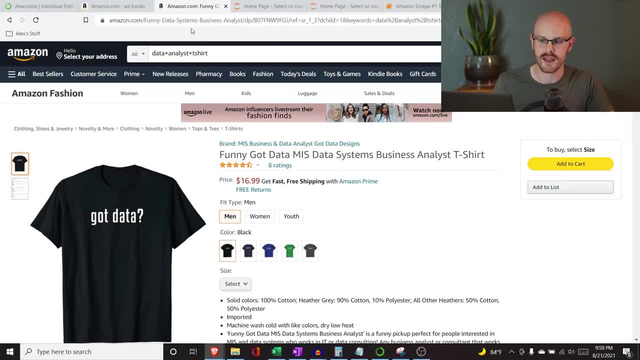 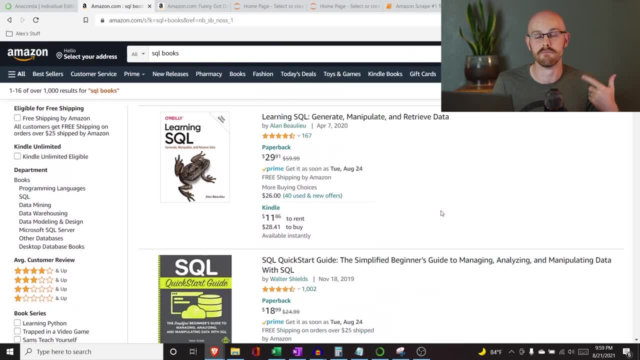 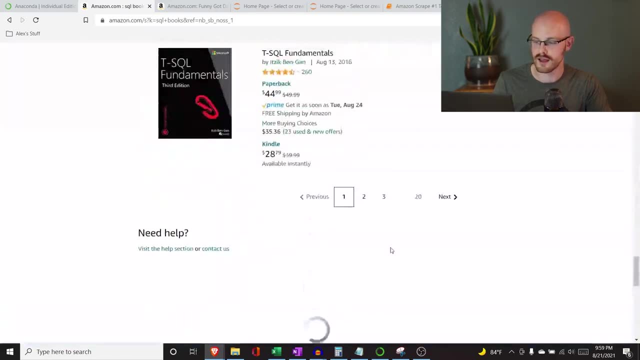 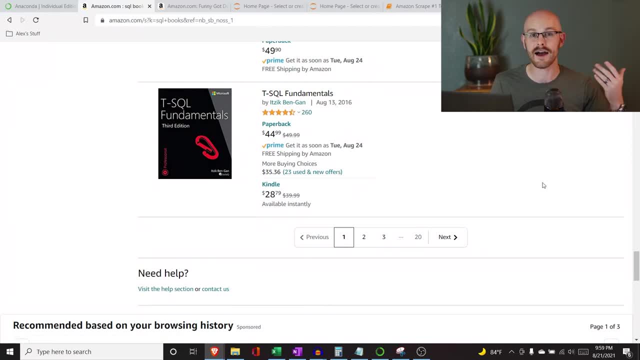 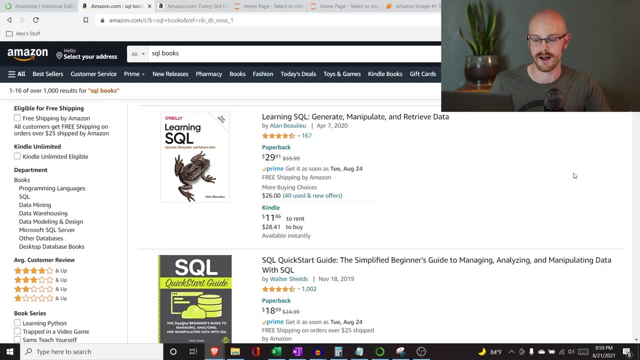 20 pages. You want all of that data. How do you get all of that? That'll be the next project. I don't know when I plan on doing that. I have it like 90 percent of the way done, but I have this one completed And so I wanted to get that out to you guys now. But that'll 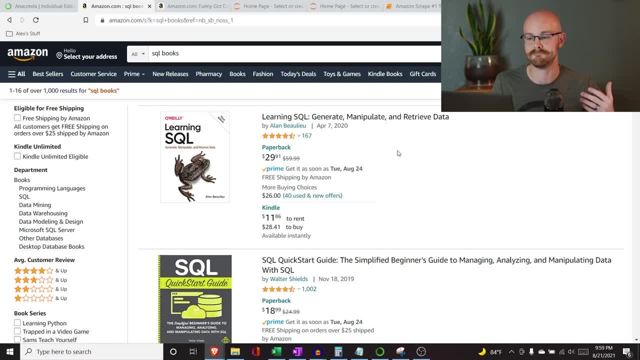 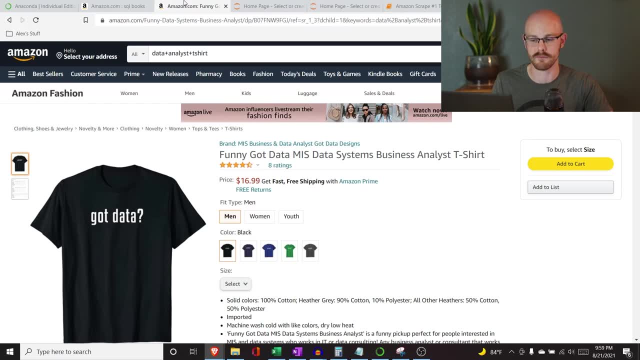 probably be the next project. I think that is much more difficult, And so if you can understand this one and you get it and you understand it, then the next project you should be able to understand too is just a little bit more complicated. So, with that being said, we are. 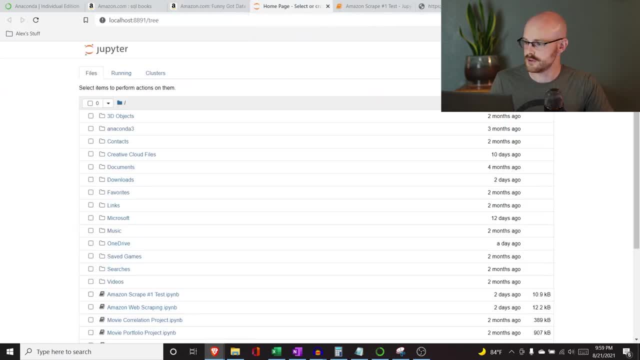 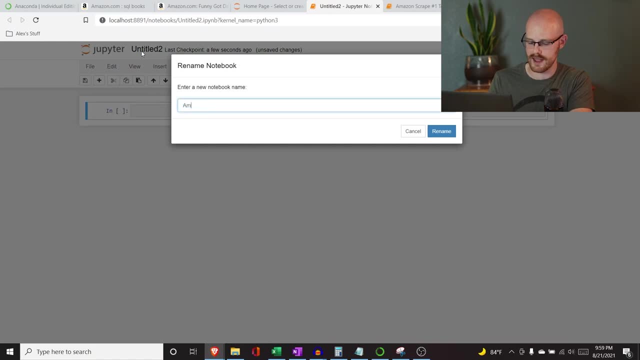 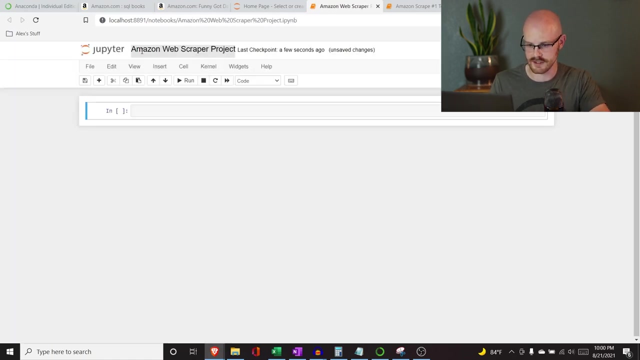 going to go to the project. I'm going to delete one of these. All we're going to do is go to new Python three. It'll open up a new one. We'll call this Amazon Web Scraper Project. That's what we'll. 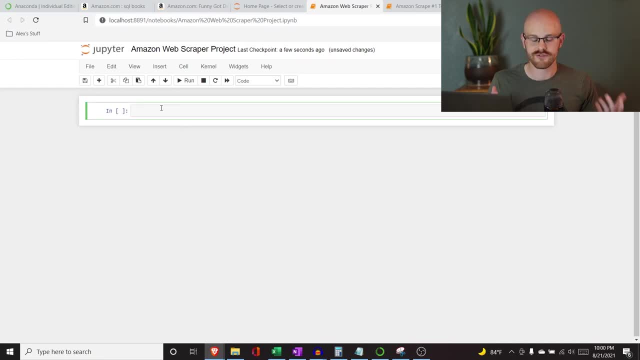 call it. I spell it right: Perfect. The first thing that we need to do, or that we should do, is upload or import our libraries. So I'm going to say import. Oops, What am I doing? It's off to a terrible start. There we go. 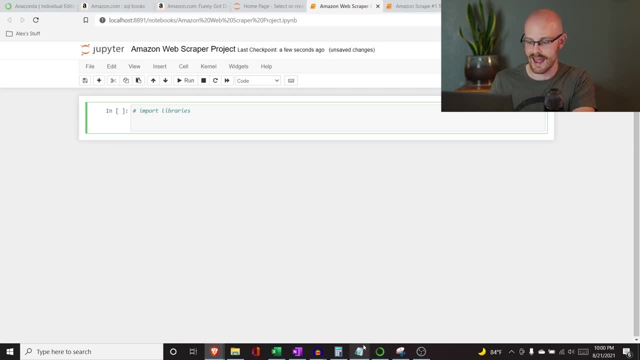 Import libraries. Now I'm not going to write out all the libraries. I have some things that I'm going to be copying and pasting throughout this. There's only a few things that I'm copying and pasting. You can take a quick glance: Some of the things that I just don't want to waste time on. 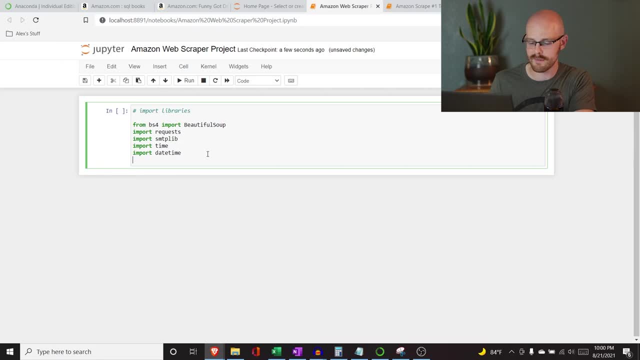 because this could be a long video. I don't know, I don't always time on stuff like this, And so you know I'm just going to copy and paste it. There will be a link below, if you haven't clicked already, that will go to the GitHub page where you can. 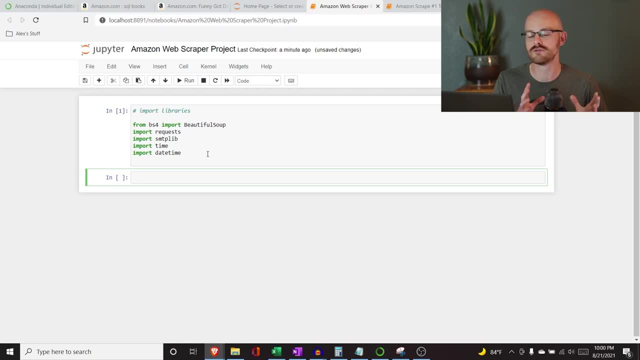 literally have all of this code already written. I do recommend writing it all yourself, because you will learn it much better, I promise, because then you'll make mistakes and you'll figure it out and all that good stuff. But you will have that code available. So just go copy and paste it, That's. 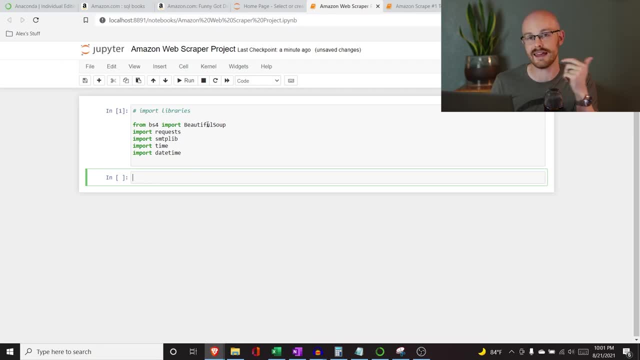 what I would do, But what we are going to be using today is something called Beautiful Soup requests. Then we're going to be using time and date time And a potential one if you want to get, and I'm going to show you this at the end. this is not really part of the 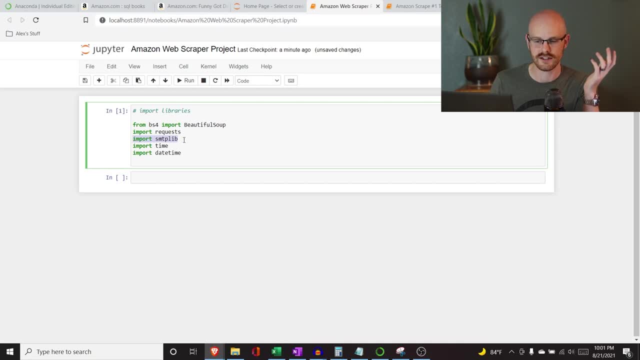 project. It goes above and beyond. But this library right here is for sending emails to yourself, And I'll show you how you can use it if you want to. I already have the whole code written out. You can just steal it and try it out yourself and see if you can get it to work, But this one is not. 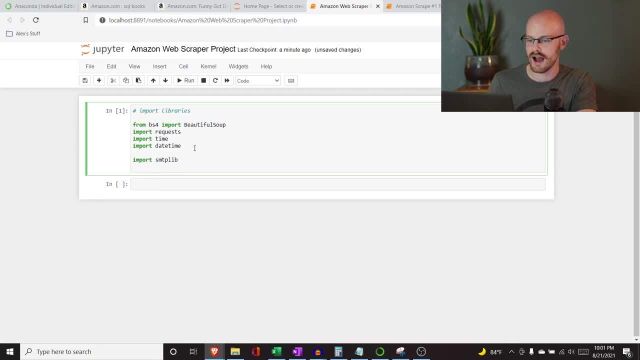 as important, I'll put it down here. So let's move on Now. one thing I want to say before we get too into it, is that, well, give me a second. Is that right here in front of me is a different laptop Now? 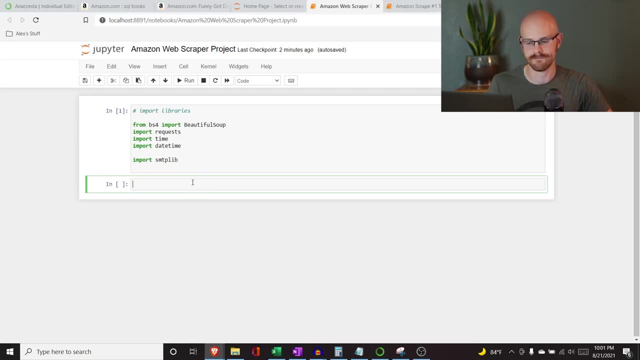 it took me a solid- I would say, you know- 10 hours or so to write all of this. It took over the course of like two weeks in my free time I'd pick it up. It took me a solid, you know. 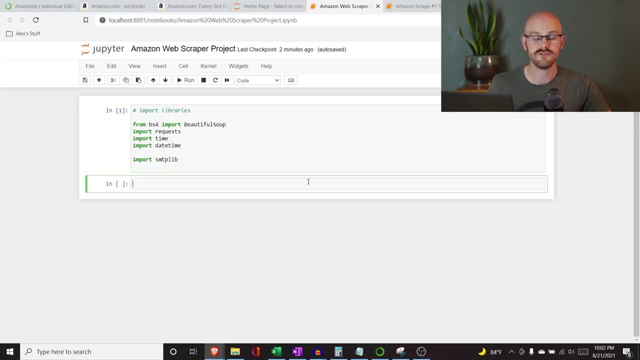 two weeks on and off, an hour here, an hour there- to finish this project, And I made a ton of mistakes and I finally got it to work, you know, after a bunch of revisions. That's typically how things go when I do projects, And so I'm about to give you a streamlined version of this, because I have all the 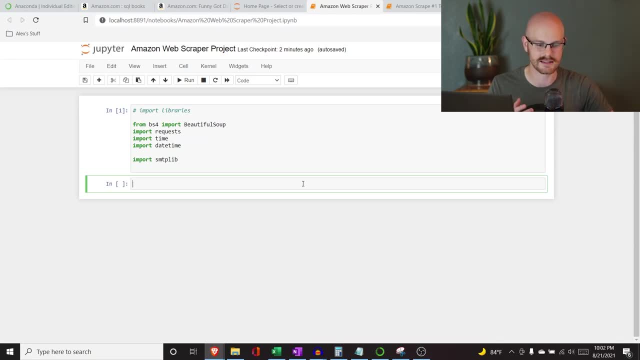 code right down here, And so I'm going to be glancing at this a lot, Just so I don't make this video 20 hours of trying to remember all the code off the top of my head. I have it written out already. I. 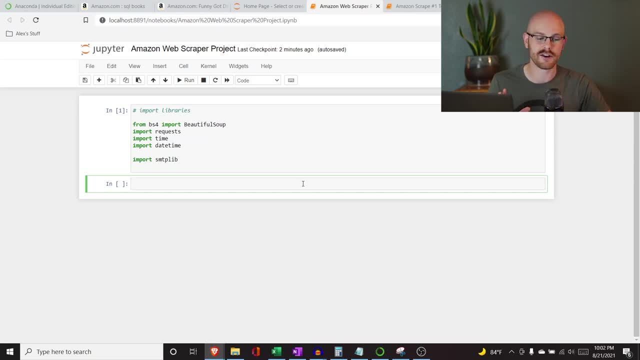 already did the project. It works, It's beautiful, It's a good project. So I don't want to waste your time And I just want you to know that you know nobody should be able to do this off the top of their head in an hour. Most people won't. It takes. 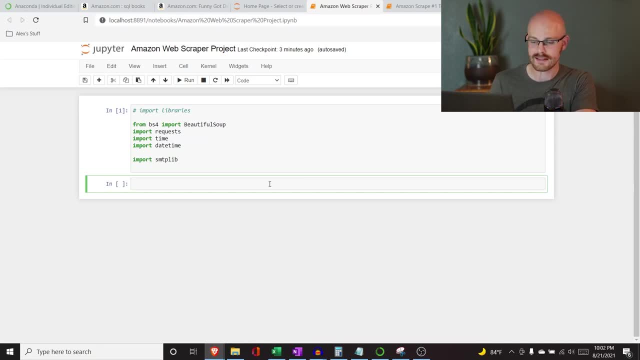 time You make mistakes. But let's get started on the project Now. in this, what we're going to have to do is we are going to have to tell Beautiful Soup and requests where we are actually getting this data, from What websites? What is our computer? You know some information from our 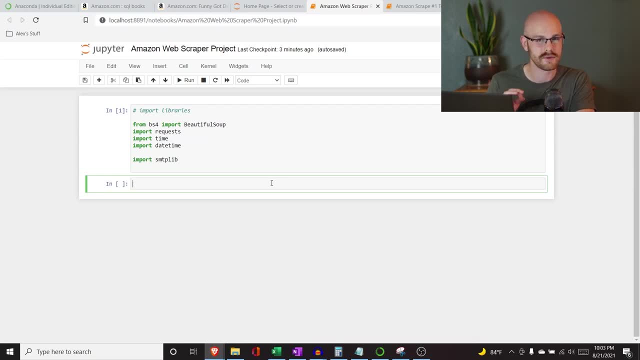 website. Again, there's going to be a little copying and pasting in here, because you don't ever, you will never, ever, ever need to know this. But right here we're going to basically connect to the website. So I'm just going to say connect to website and we're going to say URL is equal to and. 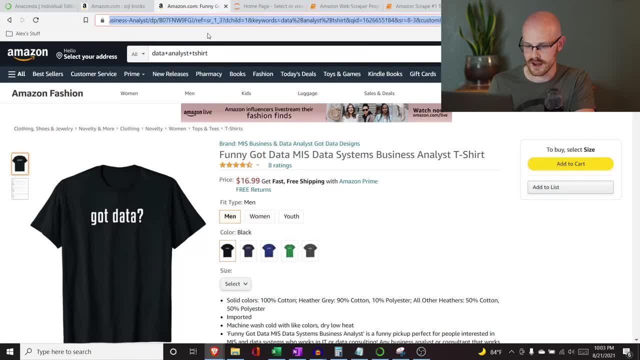 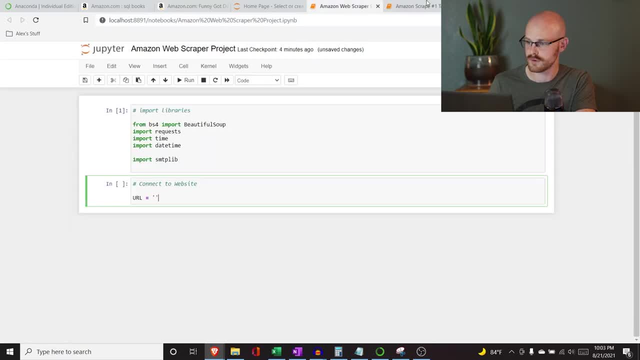 let's go get our URL. So we have this right here. so, literally, just go up here. do you know? control a copy? that, oops, That's the actual project. Get rid of it. that, uh, paste it in here and that is our url. we will use that in just a second. uh, what am i doing? 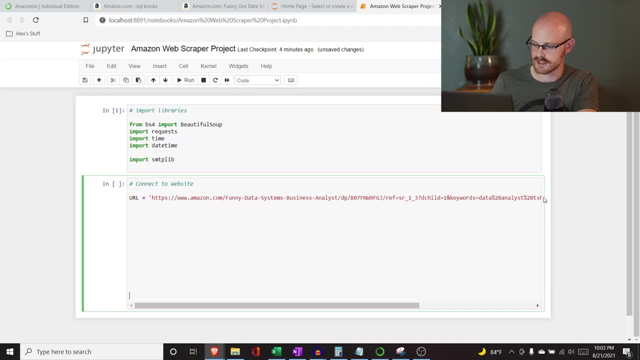 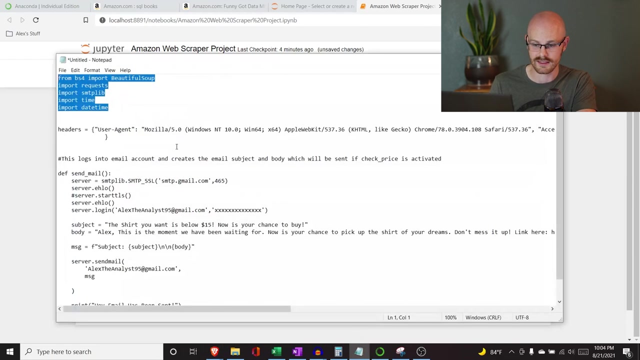 let me just get some room here. and then we, what we're going to need is something called headers. now again, you will never, ever, ever need to know this. so i'm just going to say headers. um, what i'm going to do is i'm going to copy this, i'm going to show you how to get this really quick, um, but 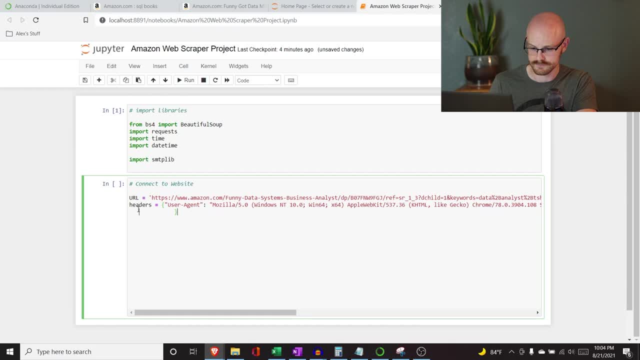 is something called headers, so let me show you how to use, how to get this and why. you don't need to know any of this. so what this headers is, is this something called a user agent? you need to do this for your computer, um, and you can do that by going to this link, right? 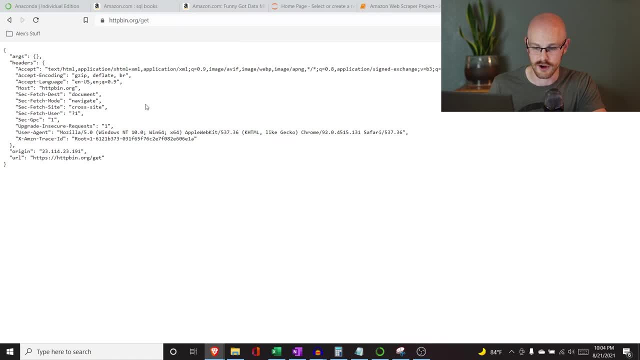 here. so i'm going to put this link in the description so that you can go and get that. and there's something right here called the user agent. so all you have to do is copy this, just like this. do copy. i'm going to go back here and i'll show you that it's. i'm going to copy it in. 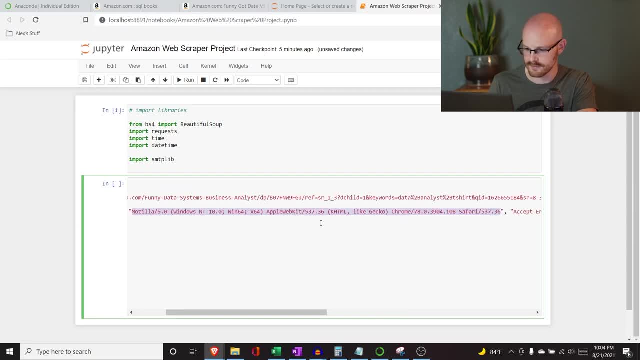 um, it'll be the exact same. so there you go, it's the exact same. um, all of this extra stuff, except encoding, except, um, this html stuff, connection close. all that. you don't need to know any of it. i promise you'll never come in handy, ever in life. actually there will be one. 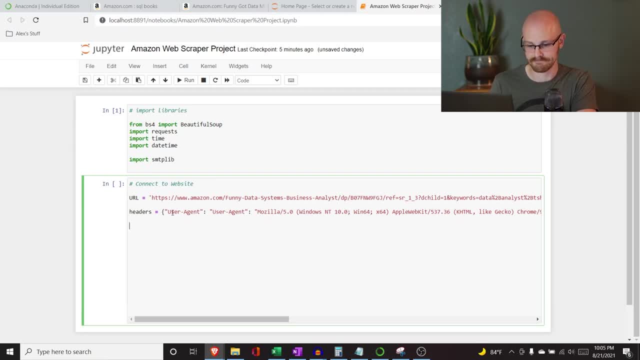 person who that becomes in handy for, and they'll be like: oh, i don't know how to do this, and then they'll message me: um, but we are now connecting um using our computer, using this url, and then what we want to write is: we want to write page. i'm going to say equals, and this is where we 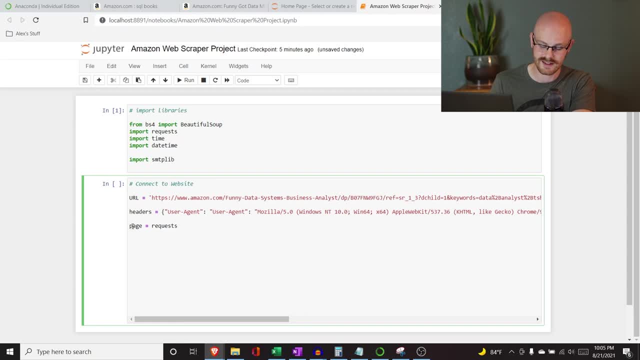 start using these libraries. so we're going to use requestsget and we are going to pull in that url and we're just going to say: headers is equal to our headers right here. so we have this And this is where we're going to actually start getting the data, bringing in the data. 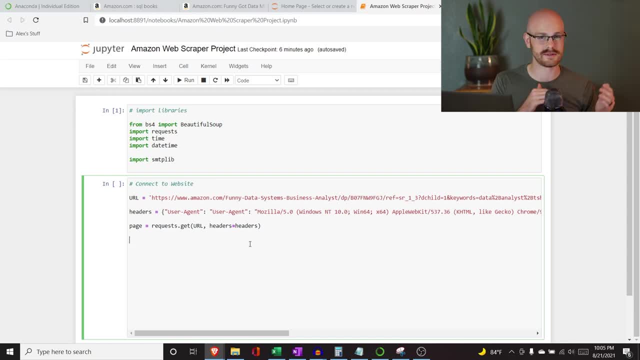 And it's not going to look like that at first, but I'll try to print some stuff out as we go along the way so that you can kind of see what it looks like and how we're going to kind of make it more useful, because it comes in very dirty when we first get it And some of the things I'm going. 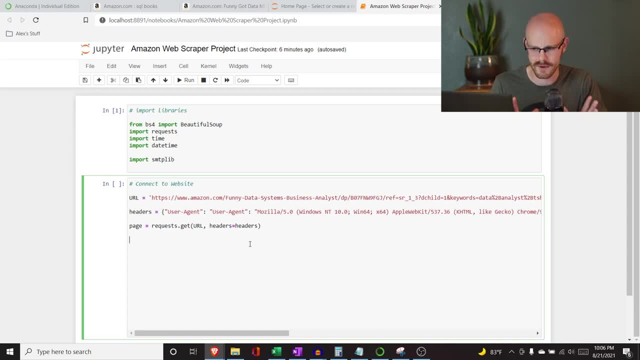 to show you will just help clean that up. And before we actually go any further, I don't want my head to be here for the entire time. I'm going to get rid of myself, so you can just see the page. I just it's less distracting. I hate when I feel like people are always watching me, So I 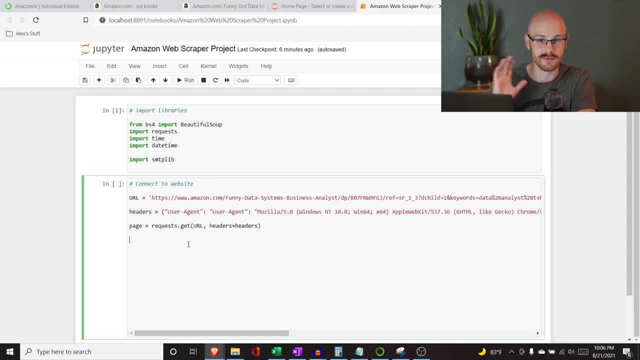 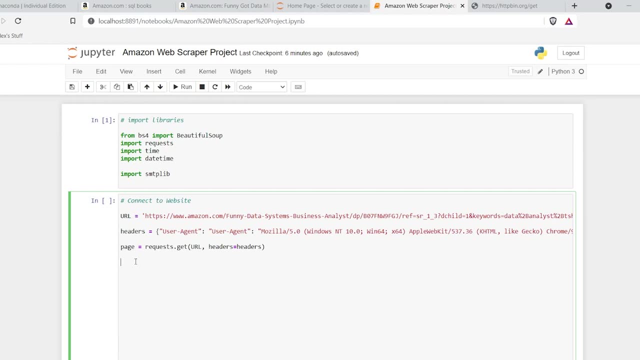 want people to just focus on the code, So I will see in a little bit. Let's get back into it, All right. So what we are going to do is we're actually going to start using the beautiful soup library, All right, So we are going to say: soup one is equal to, and this is where we actually 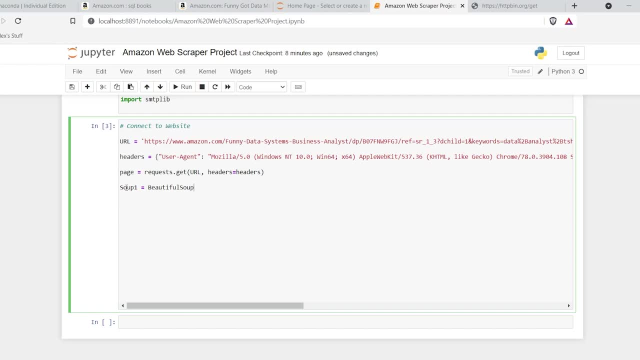 start bringing in beautiful soup. And you guessed it, You're going to say beautiful soup And then, in parentheses, we're going to do page dot content. And again, these aren't really things that you need to remember or need to memorize, We're just pulling in the content from the page. 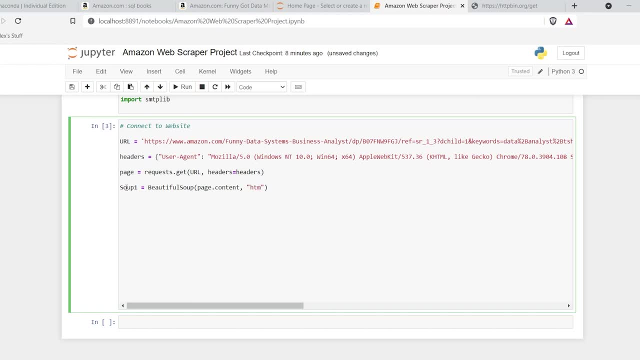 That's really all we're doing right now, And it comes in as HTML. So we're going to do HTML dot parser And let's see if I can print out. actually, let me just do soup, one I don't like. 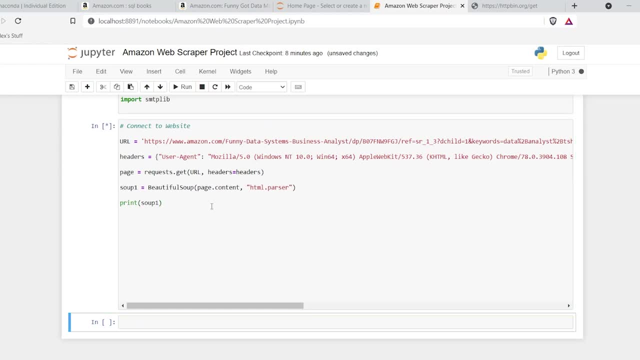 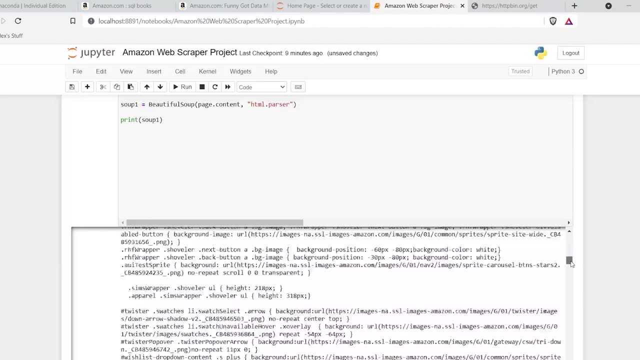 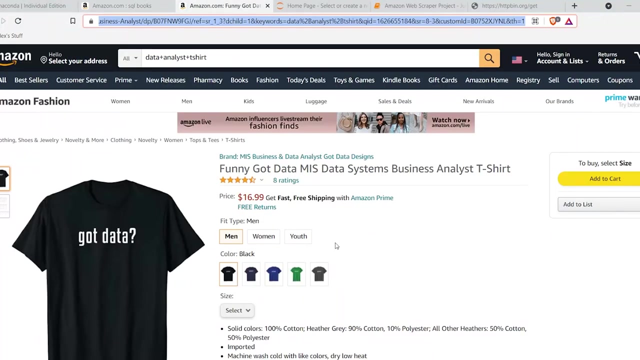 I don't like doing upper caps on stuff. Let's see if anything prints out real quick. So we are literally pulling in all of the HTML And let me go show you really quick, because we're going to get to this in a second. Anyways, if you come here, this is: this is a static page. 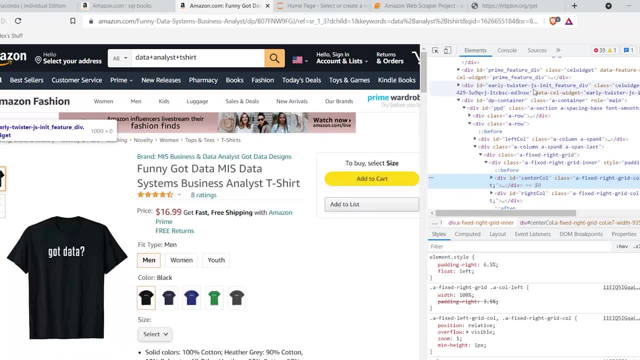 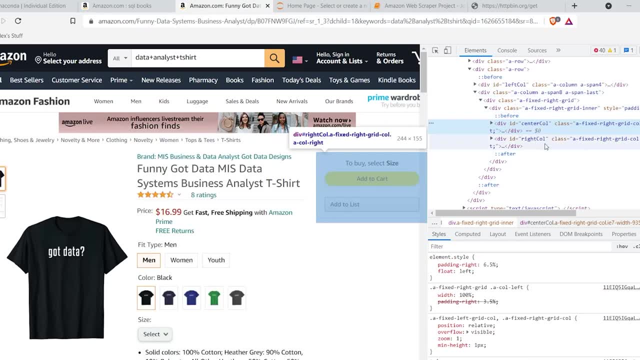 basically written in HTML. If you have never seen HTML before, you know actually, a lot of this is. you know, just stuff that most people will never use. It's just good to know. Some of the stuff is good to know. So, as you see, I'm scrolling on this right. 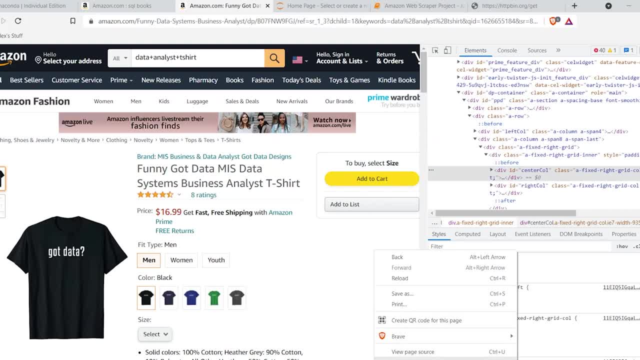 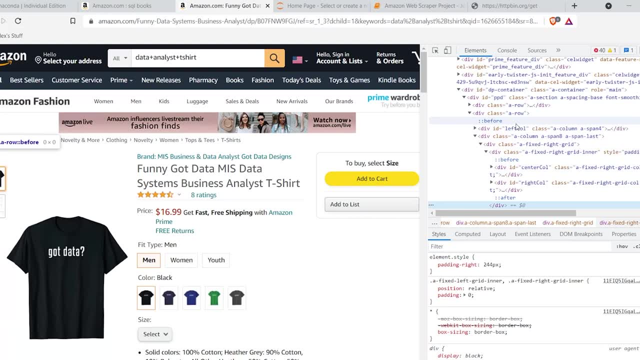 side. by the way, I did right click and inspect or control, shift I, whichever one works better for you. But as I'm scrolling over this, you should see it kind of highlighting different areas. It's hard to kind of get what you want. Let's say, we want this title. What I can do is I can click. 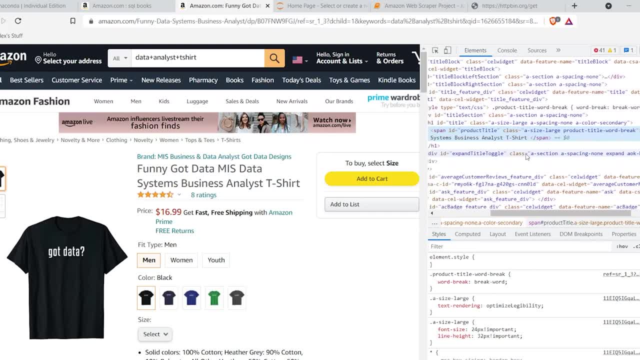 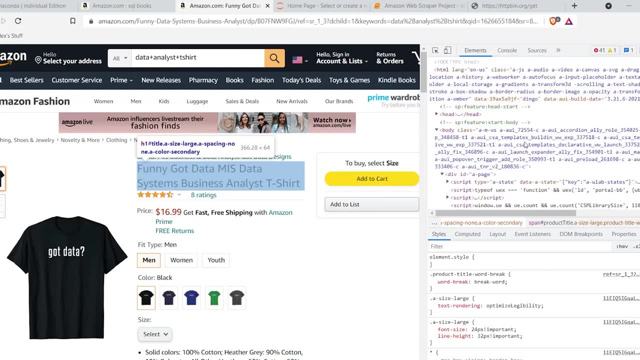 select element, go right here, And then we can select, like a type that, the header or the title of the page. Now I just want to show you, though, of what we're pulling in. So we're pulling in this doc type, HTML. all of this is coming in. 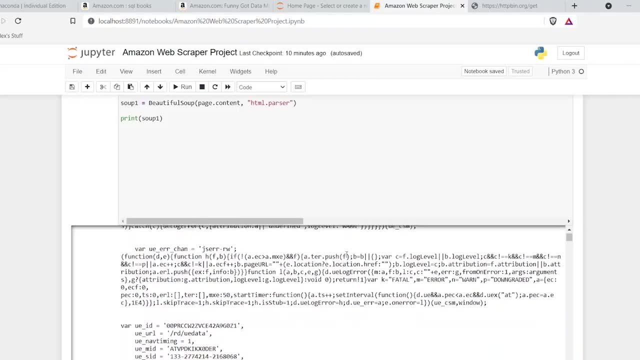 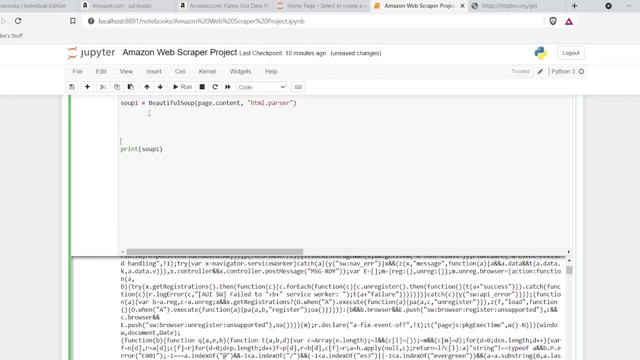 So that's what this is right here. this doc type HTML and we're pulling every single thing in. That is what we're doing right now. So let's get, or let's go down a little bit, Let's do soup. two: 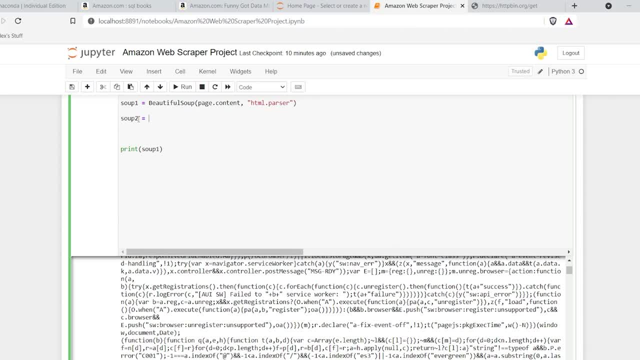 we're just going to do a very, you know, an upgrade to soup one. basically, we'll do beautiful soup again And then we're going to do soup one. So we're pulling in that content again. So that's soup one And we're going to do dot. 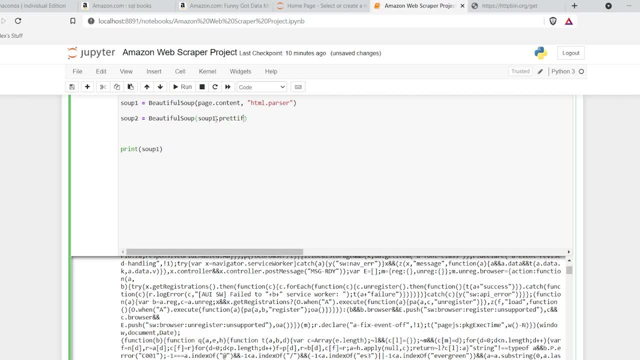 prettify. If you don't know what that is. it is common in a lot of different languages and a lot of different stuff. It just makes things look better. That's really all it is. I don't know why I'm using double quotes. I don't know why I can do. you can do single ones if you. 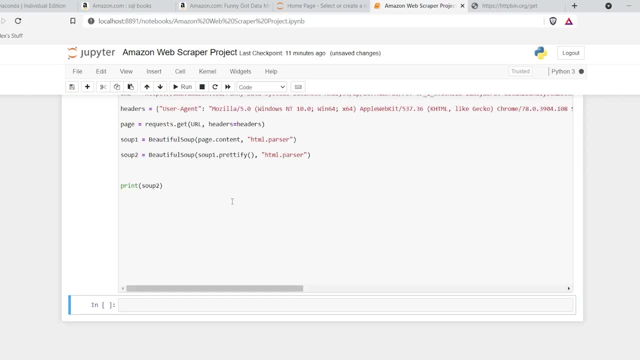 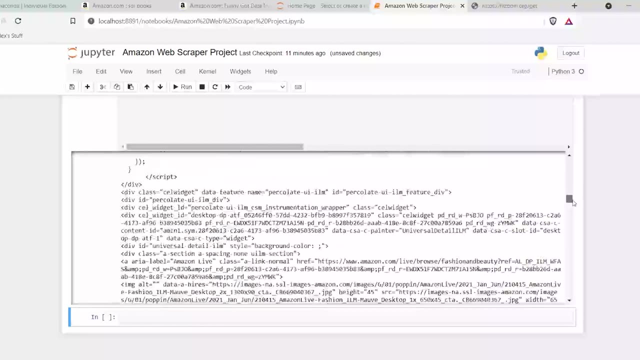 want, And now let's do beautiful. So that's what we're doing. So let's pull that one in, Let's do soup two, And it should just be, it should be better formatted, And let's see if that's true. And it is so before, if you did, if you can. 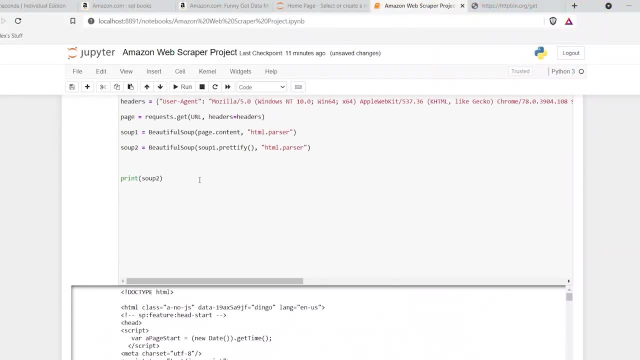 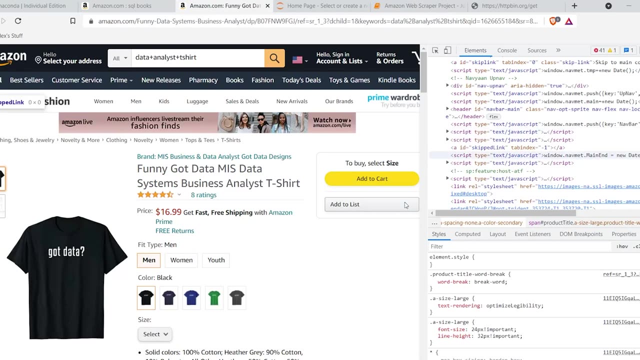 tell it was, it didn't have basically any formatting, has a little bit of formatting now. it'll help in a second And you'll see that. But now what we want to do is go back and want to actually get the data that we want. 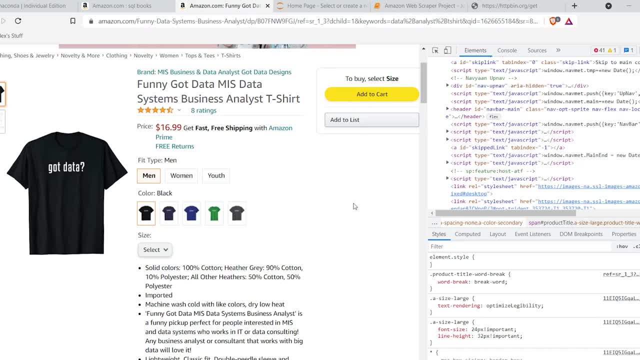 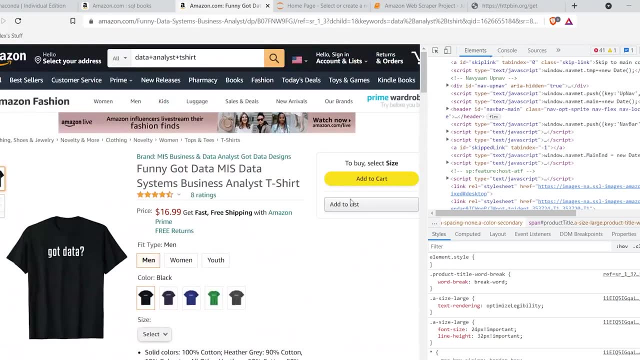 Now you can get any data you want. I'm going to show you simple things, easy: Um, in my, in my, in my opinion, it gets more difficult the more complicated stuff you start pulling Um and and you'll understand that as we go into it. So what I'm going to do, 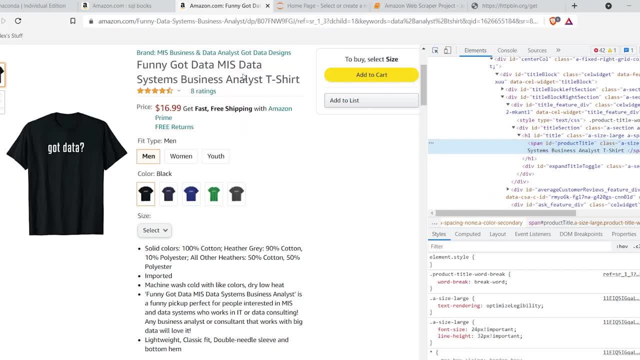 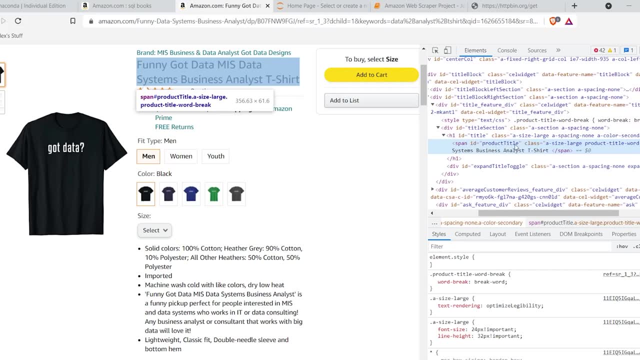 is: I'm going to select this and I'm going to select this um the title. I want that, And so if you do span ID, it's equal to product uh title. So we need to remember that. um class. 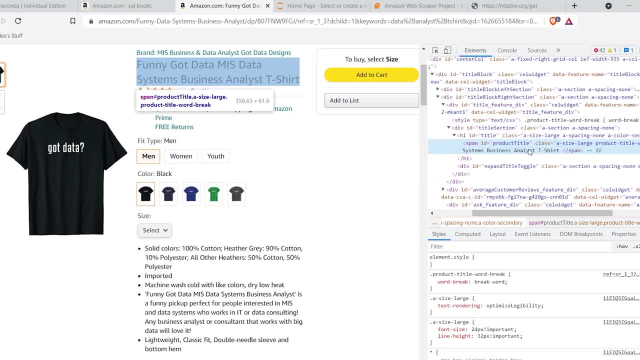 we don't need to know class, I believe. uh, we're going to be using that ID. this um ID equals product title, So that's what we're going to be using. Um class will come in in the next video. 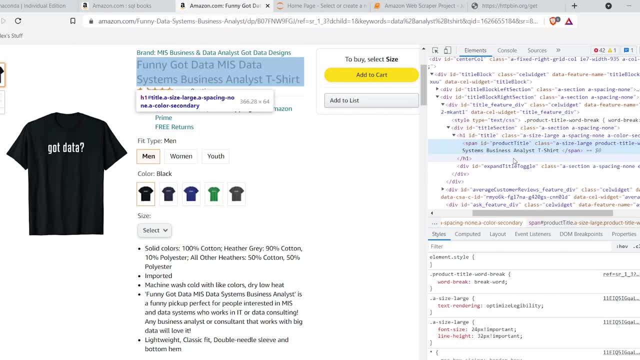 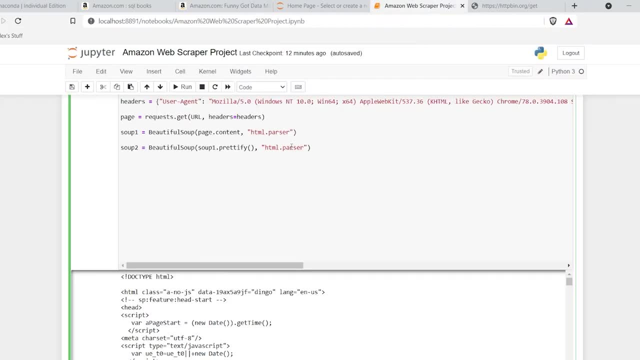 And we start looking at these: uh, but not in this one. So let's remember, ID equals product title. So let's go back over here. So we have this soup too. It's basically all of that HTML in it right down here. That is what we were pulling in, So we need to kind of specify what we 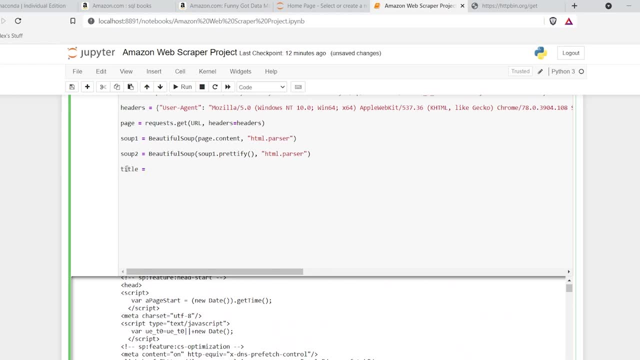 actually want. So let's say title, That's what we're going to be getting, Um, and we're going to do soup too. So, using, taking all that content, um, and we'll do find and we're going to do open. 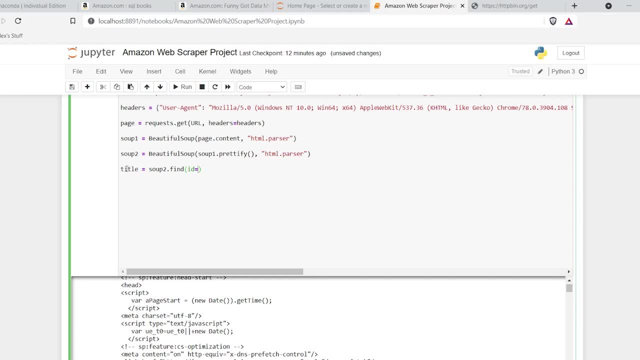 parentheses And we're going to say we want to find that ID where it's equal to product title, And then we're going to do dot, get underscore text, And then we're gonna do open parentheses. So now let's um, let's print. 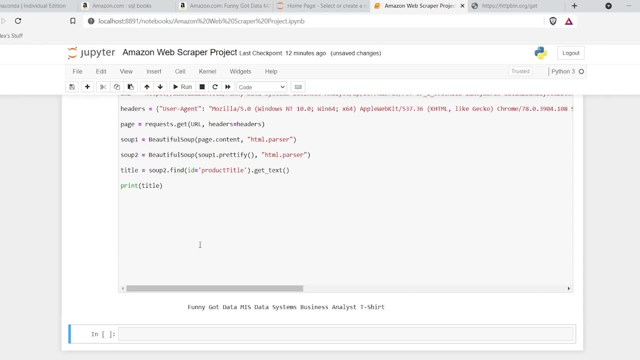 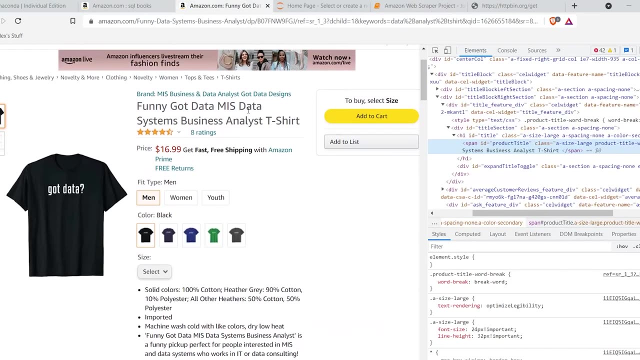 The title and see what we get. All right. So that is exactly what we're looking for. It's funny: Got data MIS um t-shirt. that that is what we're trying to pull in, So that's perfect, That's. 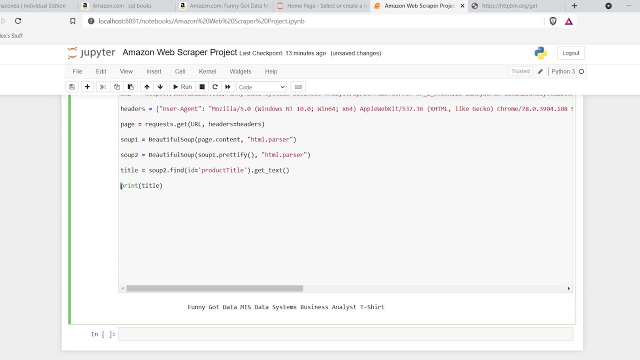 exactly what we want. We don't. uh, let me, let me just do this, Save me some time later on. We don't only want the title, We are also going to be pulling in the price. So if you can guess, uh, we'll be doing some. uh. 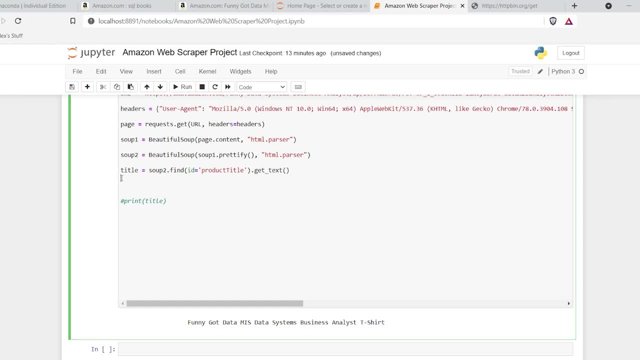 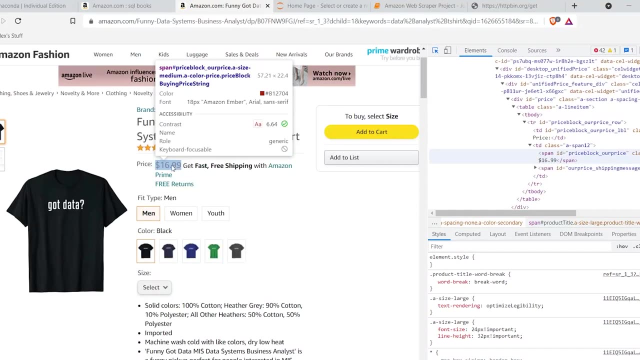 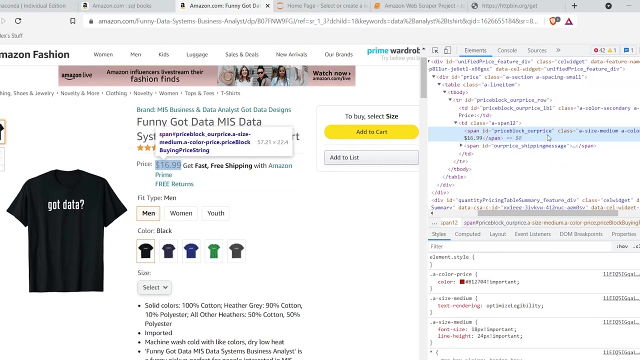 a data set on the actual pricing, Um and so let's go back here, We're going to again use this right here and we're going to go to this price. And it says again: we're going to look at this ID. The ID equals price. block underscore our price. So fairly easy. 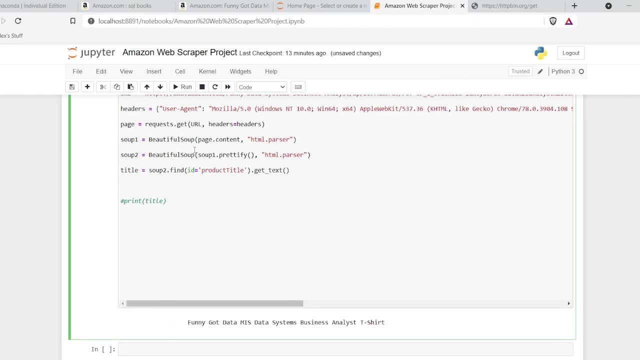 You can copy this, I'm just going to write it out: Um, we're going to say price is equal to soup, to find it's going to be again id is equal to, and then it's going to be price block, underscore our price. 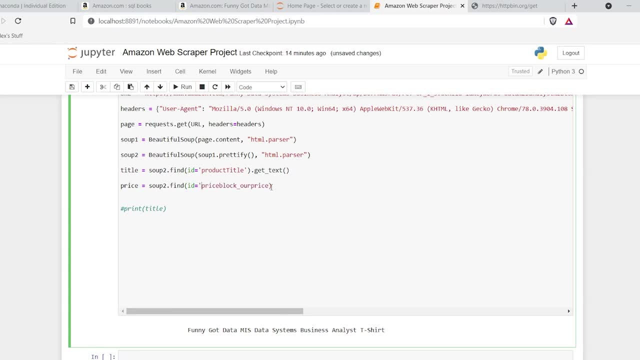 and i saw that right, excuse me. there we go and the exact same thing: dot, get, underscore text, parentheses. uh, and there's a get text, there's a get all or get all text, um. so you know that get text is a specific thing that we are using you we might use a different one later on, um. 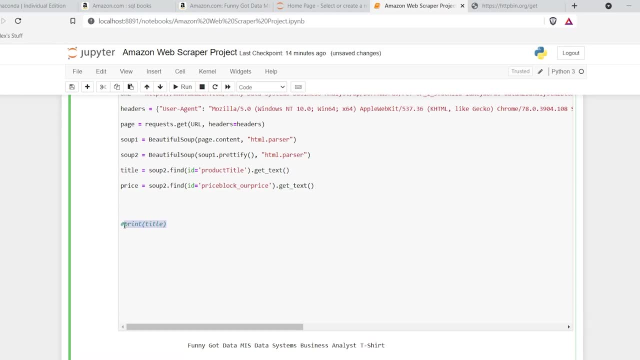 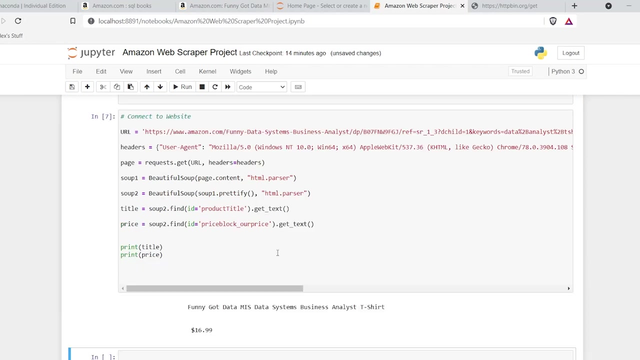 but that that is what we have. so now, let's let's print the title and print when i, when i have all this too much, uh, too much space. so let's print the title and print the price. now let's see what we get. okay, so we have our title and we have our price. i mean, you know, i don't know what all this. 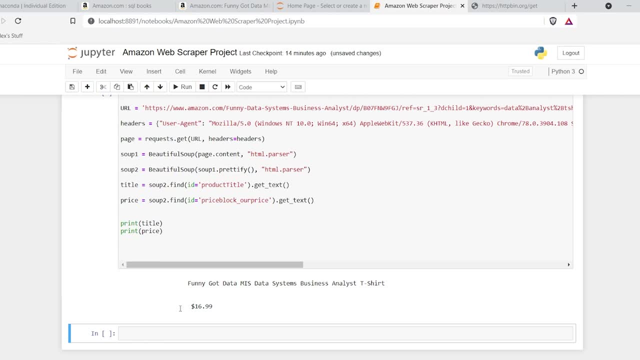 white space is, but i don't know what it is. but i don't know what it is, but i don't know what it is- is over here, um, but it looks like there's a lot of white space over here. we'll have to get rid of. 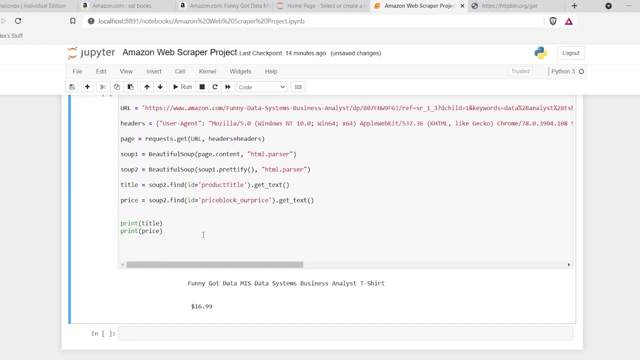 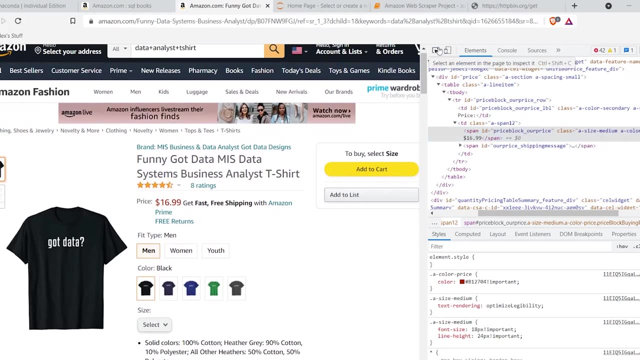 that, uh, in a little bit, as we clean it up a little bit, you can, if you want, do things like: um, you can get, and this is up to you. i'm not going to do this right now, but i'm just going to show you how to do. 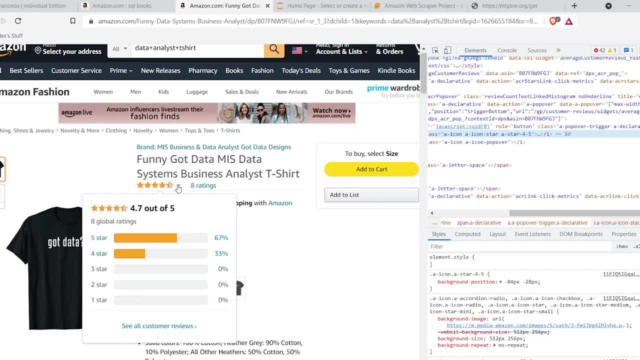 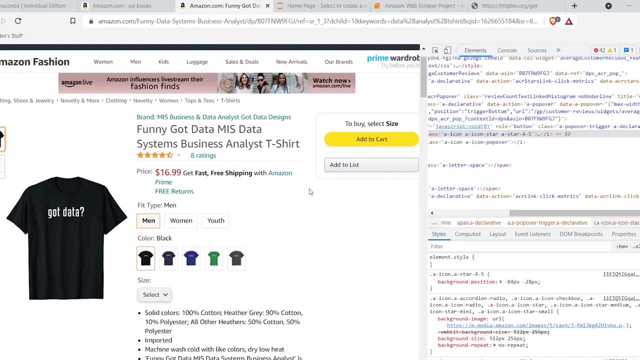 it. you can get this where you're pulling in the ratings, um, which is, you know, if you want to look at, like, how the ratings over time or or what ratings are for specific products that could be really useful, um, you can pull basically anything. you can go down the product details. 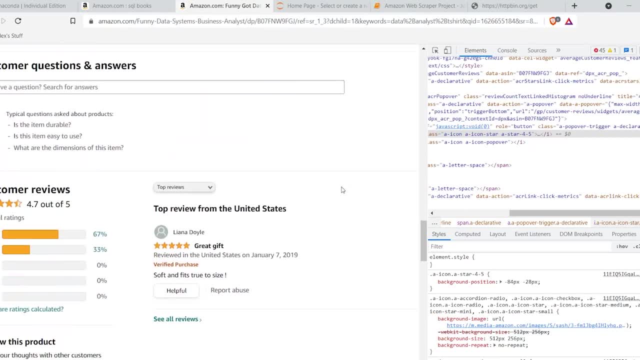 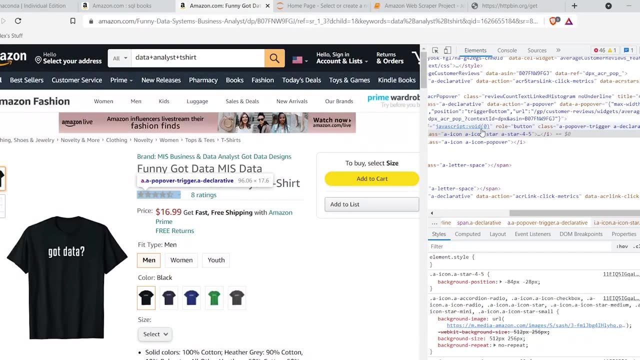 and look at dimensions, anything you want on this page. it is static, so you can go in here and pull anything it's. you just have to pull it from the html, know where you're looking, pull it in, um, and now, when we go back here, excuse me, i'm going to show you now kind of how to use this. 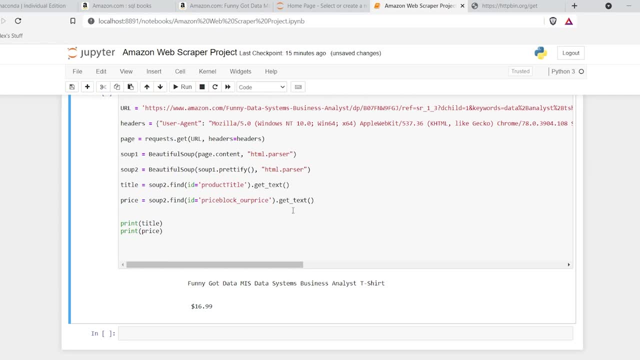 right because we have this, but how are we going to use it? that's kind of the important part. i think first thing we need to do is clean this up a little bit, because it just is. you know, if we try to use this, it wouldn't be super useful because it'd be. it's just a little bit dirty, it's not? 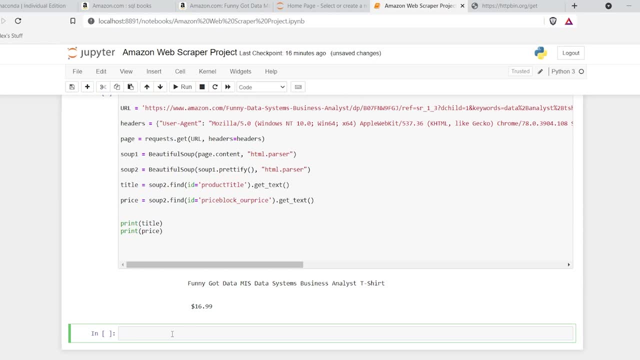 super clean, um. so what we want to do is: let's start with the price. why not? we're gonna say price dot, strip, um, and that's just going to take, uh, basically the the junk off of either side, and so let's run that real quick. so this is what we have, but what we can also do is: i don't want. 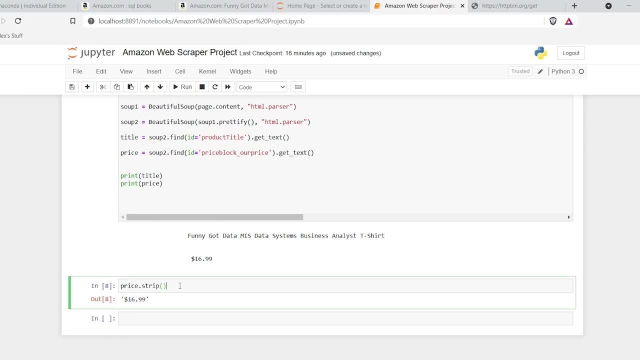 that dollar sign. i just want the numeric value. later on we are going to be putting this and we are going to be creating a process to put this into an excel file. again, we're trying to create a data set. i don't want you to have to copy and paste stuff. this is all going to be automated. 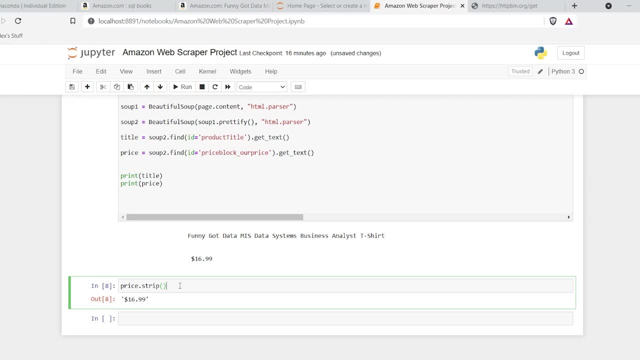 basically to input this data into an excel file for you or a csv file for you. so you know, think about making it useful in a csv or in an excel later on. so what we can do is do a bracket, and we're going to do one, and then 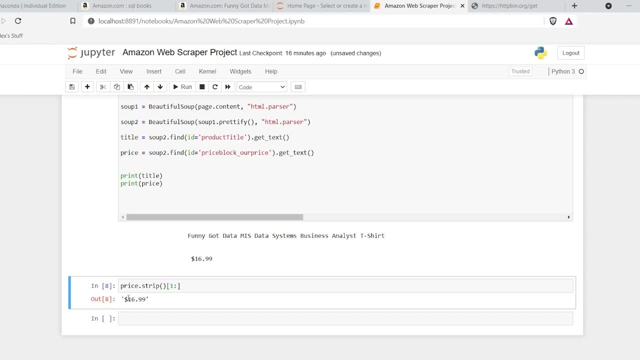 everything after that. so basically, it's just going to take everything from the first position onward. so let's run that and there we go. so let's just say price is equal to price, dot, strip, um and pull, uh, just do everything after that first, um, that first, not value. what am i saying? 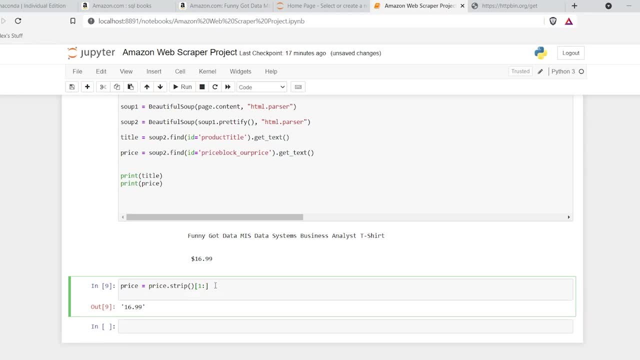 what's the word for that? i can't remember the word. the first space. that's not the right word. but all right, let's do the title. uh, this is basically going to be the exact same thing. i'm super easy, so we're just going to do title: dot strip. 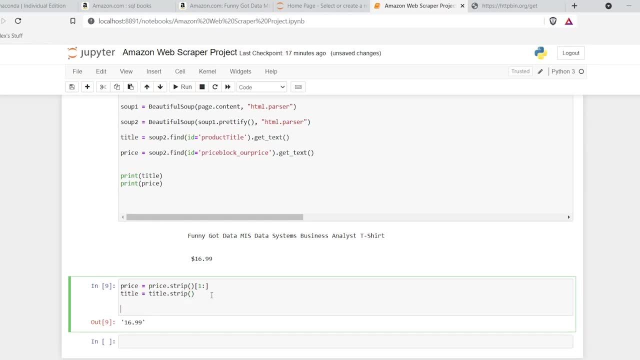 and open parentheses, um, and we can you know if you want to do this exact same thing. so now we have it, it's a little bit cleaner. so this is what it originally looked like, and now this is what it looks like. so you know nothing super crazy, but you know something. 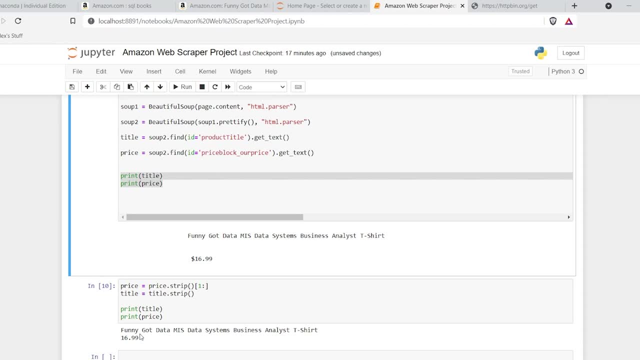 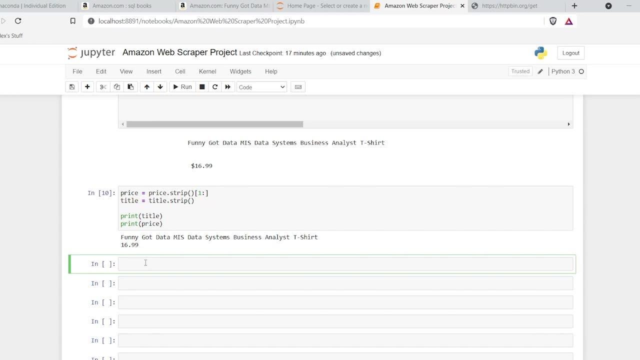 to know, now we are about to, in the very next part, what we are going to do, and let me just add a few of these because it makes me feel better. um, what we are about to do is we're going to create our csv, to insert this data into the csv, and then, later on, what i'm going to do is show you kind. 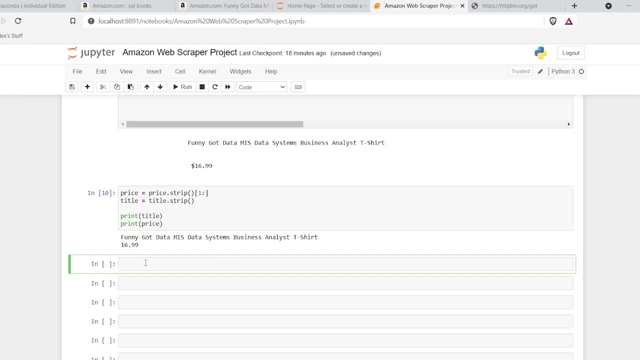 of how to um automate this process, to pull this data, um to create a data set. right, just pulling this one time and putting it into a csv really doesn't do anything. you can just copy and paste it and save yourself a lot of time. um, what i'm going to show you is is um basically doing it. 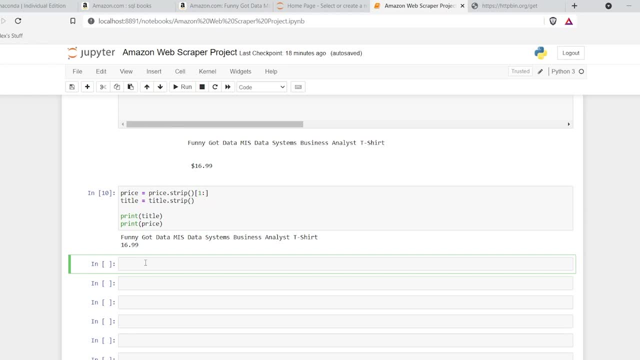 over over time and just having it automated in the background. that is what i'm going to show you. um, i guess a spoiler, but what we need to do is we need to create- uh, create the csv, insert it into the csv and then create a process to append more data into that csv. um, i'm doing a lot of talking. 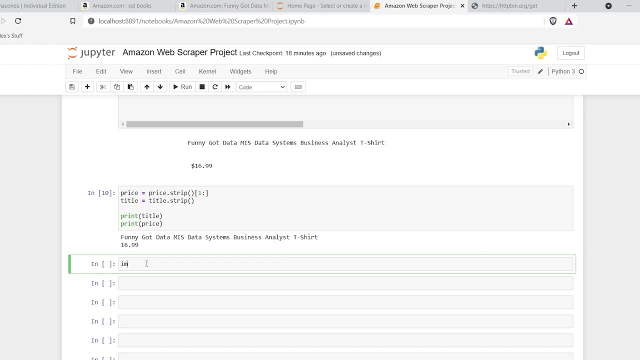 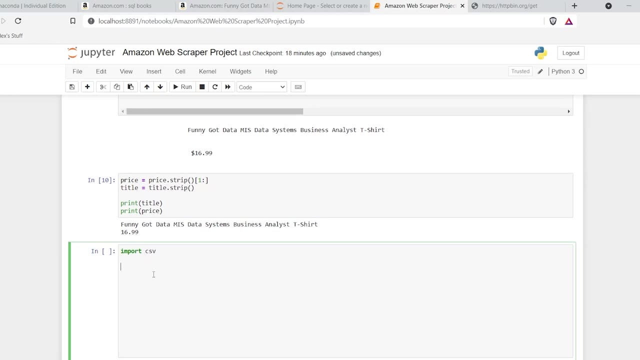 let's do some writing. so we need to do is we're going to use um. i should have done this at the top. maybe i'll go back and add that later on. we're going to do import csv now in a csv. what you want is you want. 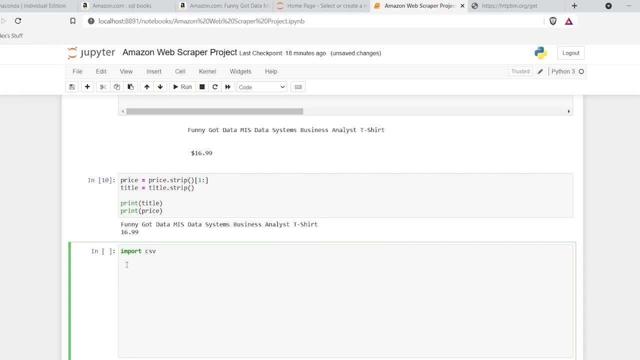 headers. and then you want the data right. so for our headers- and we're going to call it header- we're going to do um, we're going to do a bracket and let's make the first one a title, because that's going to be. we can call it title, you can call it product, whatever you want. i'm just going. 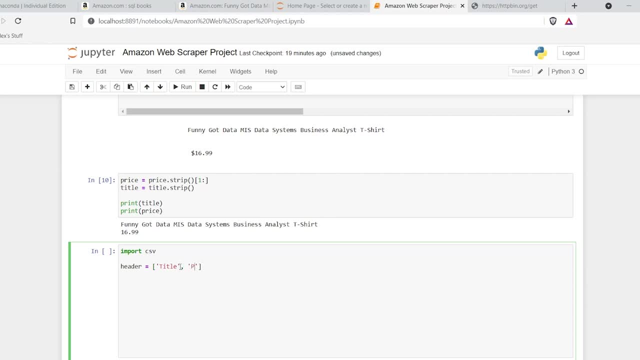 to call it title and then we'll also have price. now we need our data. so i'm going to say data is equal to now. this is important- um right now, how our data is, and i can do this right here. we're going to type um title or no. let's do type price. so these are strings and that's important to know. 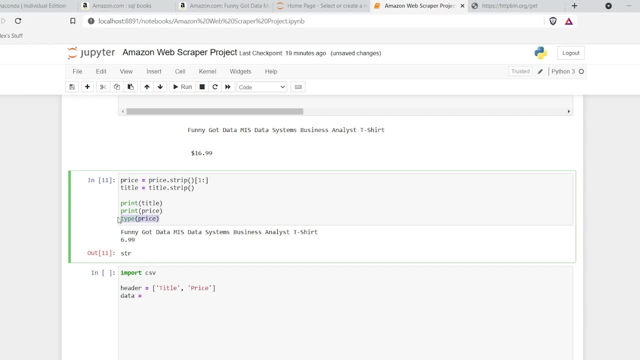 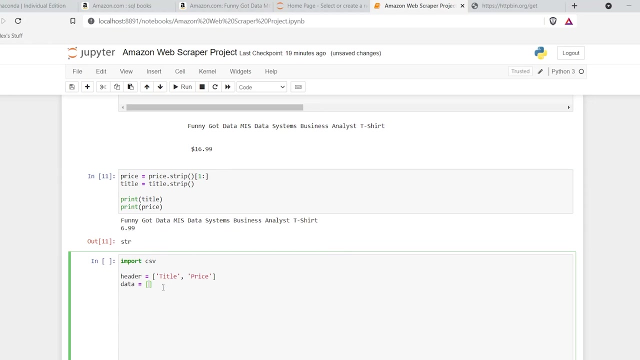 um, again, i don't want to get too much into, you know, dictionaries and arrays and lists and and strings and all these things, but this is a string and you can't put that right now. it's not super usable. what we're going to do is make this a list, um, and so i'm doing an open bracket and i'm 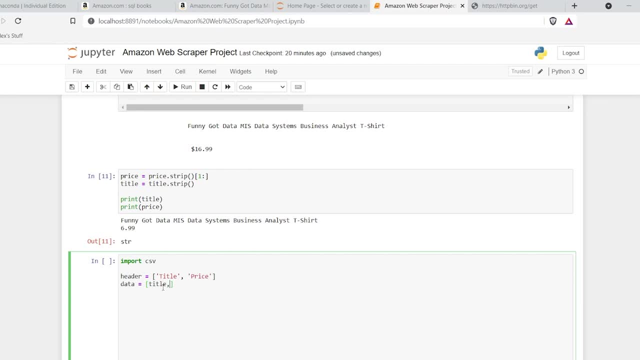 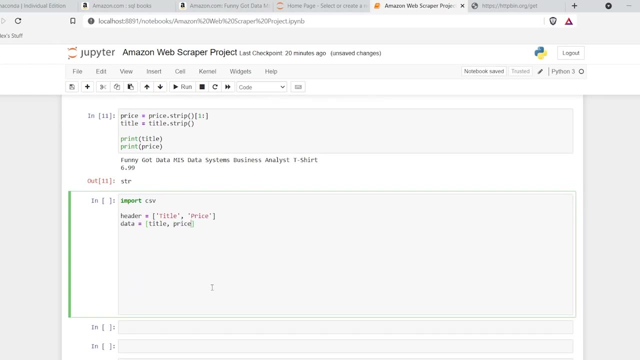 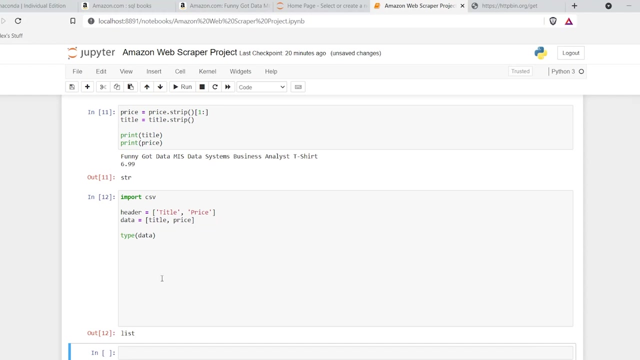 going to say: our data is title comma, price: oops, price now oops. if i do type oops of data, i'll just run that it's a list now, um, and this is important because you can run into a lot of issues with this stuff. it's really 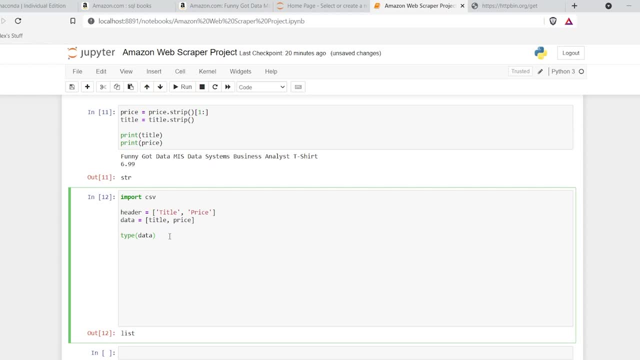 important to remember what's what type um, how do i say this? uh, how your data is. is it a list as an array? is it a dictionary? um, you know what is it. these things are important. they do play a big impact, especially with this type of stuff, so just want to show you that really quick. 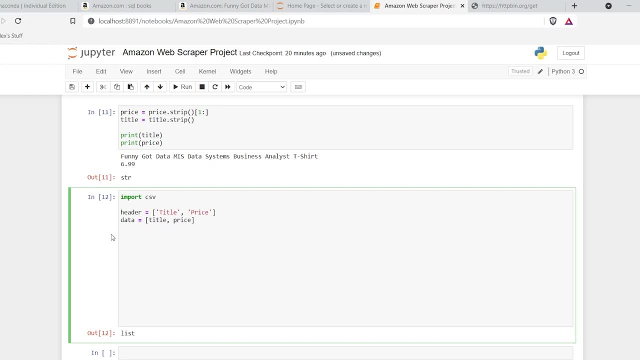 but what we are now going to do is create a csv. you're going to create an excel. i call an excel csv, you know whatever you want to call it. so what we are going to do is we are going to say with and we're going to say open, and now we're going to 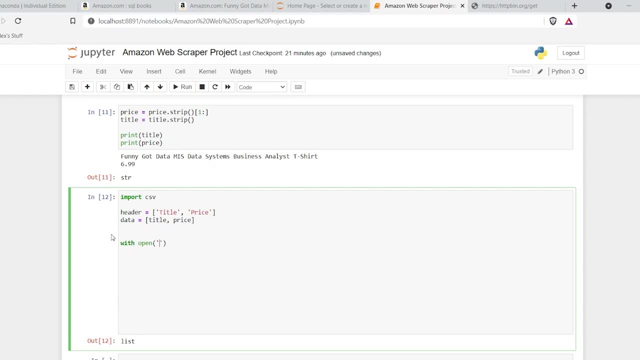 name our file. you can name this whatever you want. i'm going to call it uh, um. amazon web scraper data set- that's real long- dot csv, and then we're going to do underscore w and that means right, um, oh, whoops, that's not right. just like i was wondering why that was uh. 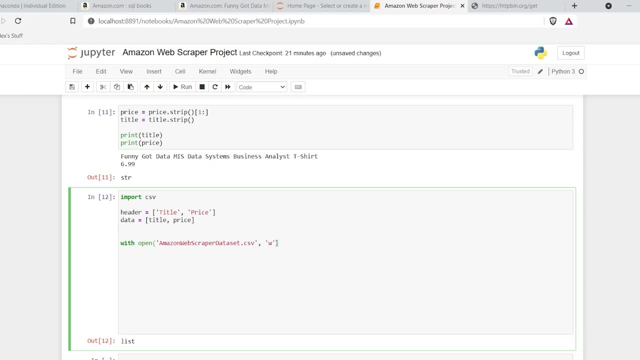 in black, uh. so we're gonna do w, which means right, um, and then we're gonna do new line. if you don't know what new line is, uh, all that does is when we insert the data, it doesn't have a space in between each csv. and then we are going to do: encoding is equal to. 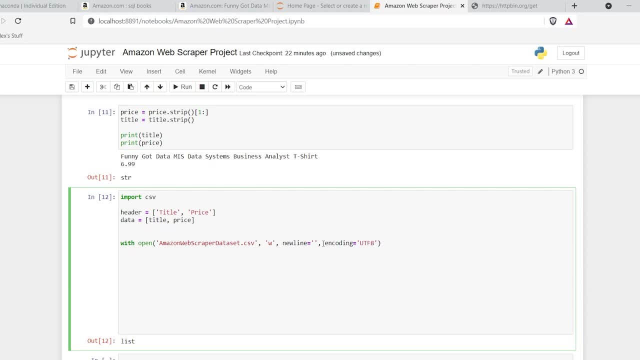 is equal to utf8 and that is it, and we'll just say as: uh, let's do f. so some of that stuff you don't need to know, some of it's useful. this w definitely need to know. this new line is is good to know and, um, i'll take it. i might take it out just to show you what. 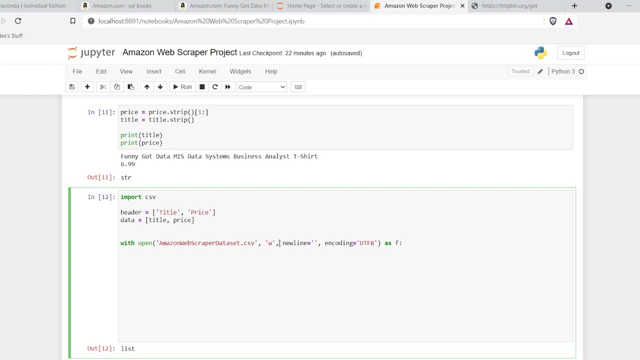 it actually does, because it's annoying if you don't have it. i promise um, but you know that that new line is important. this encoding, you know good to know- i think that's my default- is- is it's like that? uh, anyways, what we're going to do now is we're going to: uh, it's something within the csv. 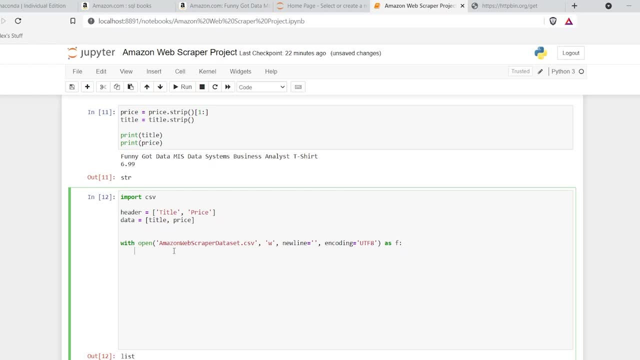 within the csv um library. so we're going to do something called csv writer and- oops, csv dot writer, and we're going to do open parentheses and that is that, and we'll just call that writer and then we'll do: this is where we need to actually create the heaven, and there we go. so i did, everyone do. anything else that we need to do everything else. i did everything else i did. i'm bad, so did. let me just bring that more, and i kind of need to like generate tidest facilitators. okay, i needed each of which iand i have boatай to take care of a second here, so i'm going to create what is called the. 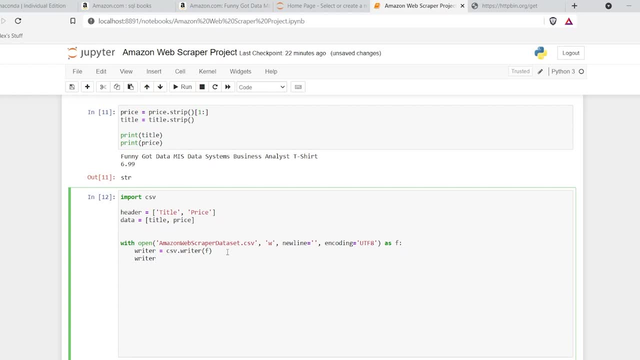 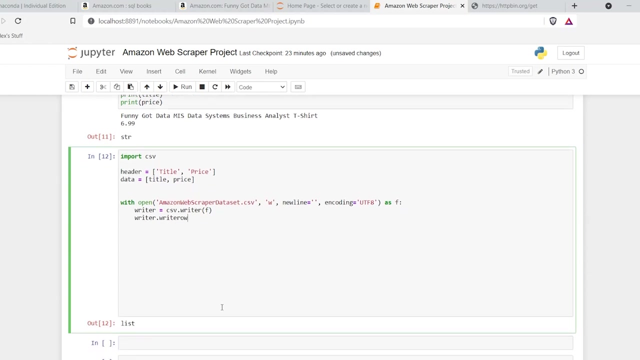 so we're gonna do: writer is dot- sorry, writer dot write row. and this is just for the initial, the initial import or not import, the initial insertion of the data into the CSV. this is what's important. the next one that we're gonna write is for when we're actually appending the data, which is gonna be a. 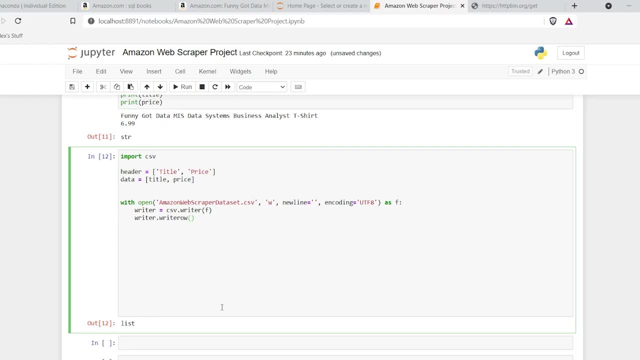 little bit different, but anyways, we're gonna do write row, open parentheses, and this is where that header is gonna go. so we're in it that these headers are gonna be the title and the price, and then for our last one, we're actually write the data, which is this data right here, and we're gonna say: writer, dot, write row and. 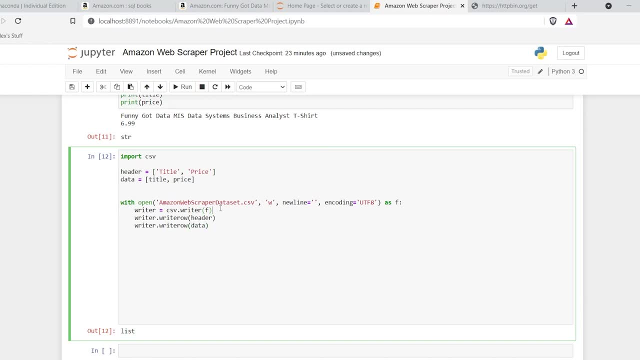 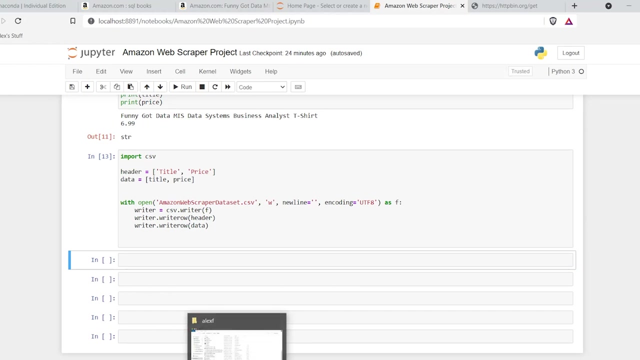 we're gonna do data, so this one: we are creating the CSV and then we are inserting the header and inserting the data. so super easy. yeah, I think that's fairly straightforward right now. let's do this and let's see what happens. so I just ran it. let's go over here and here somewhere, Amazon web scraper data set. let's open. 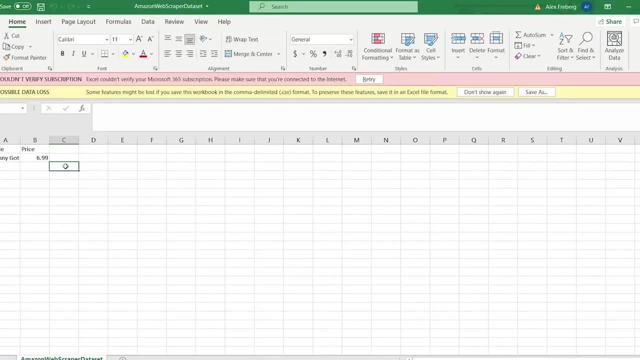 that up and there we go. oh geez, this isn't good. can't verify my data. I can't verify my data. I can't verify my data. I can't verify my data, my subscription- why does it say $6.99? I'm gonna go back and look, but I think I 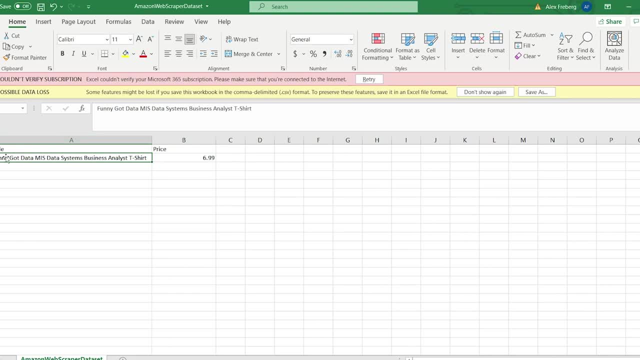 know the issue, but this is exactly what we want now. of course, we want more data and maybe a little bit more useful data, and I'll show you how to get that in just a second. but we just created that out of thin air. that was not. I didn't. 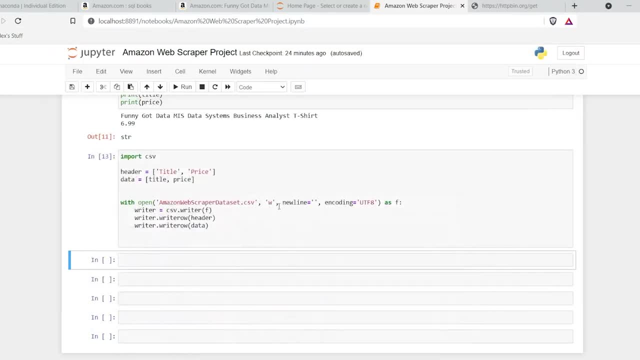 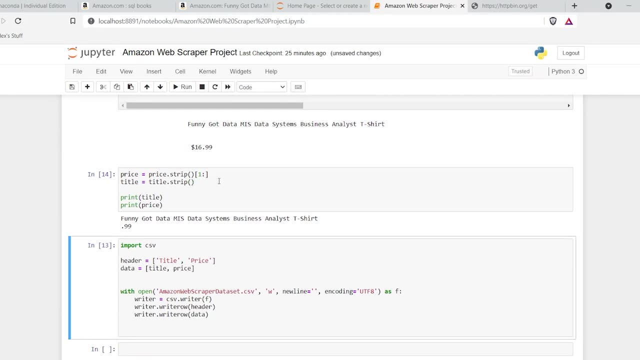 have that saved before. so we have this data set and the issue was is that I ran this multiple times, so now it's $6.99, if I do it again it's $99, and if I did it again it's yeah. it gets rid of everything. so I'm just gonna run this again. run this. 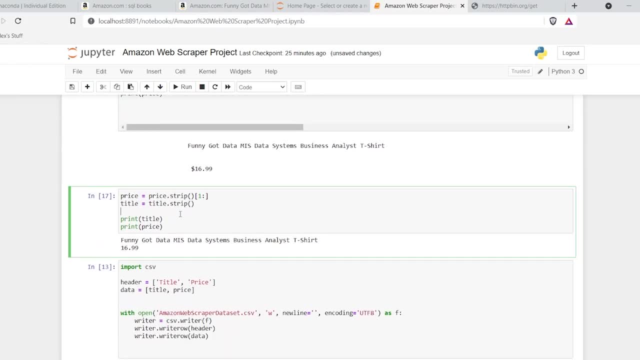 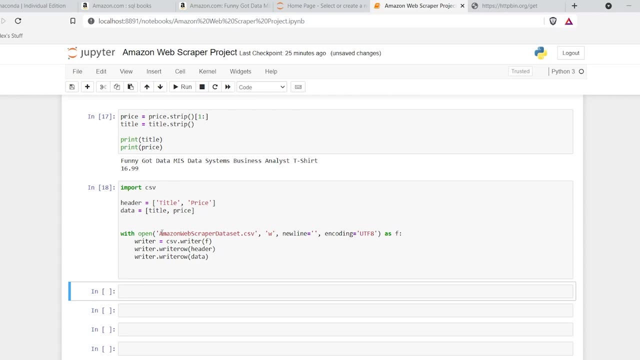 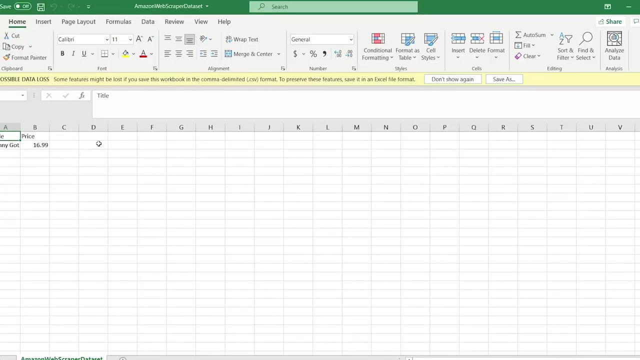 again. now everything's back to normal. okay. so now, if we run this, it's going to overwrite this Amazon web scraper data set CSV and it will put the data in properly. so there we go. oh geez guys, this is embarrassing. I'm just kidding. this is absolutely amazing. 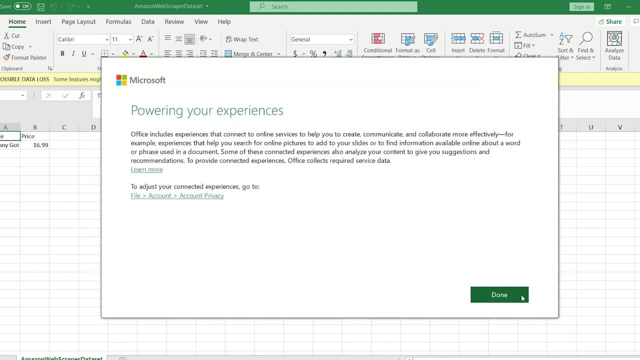 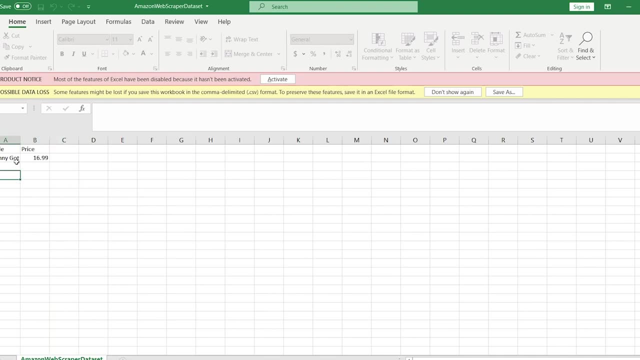 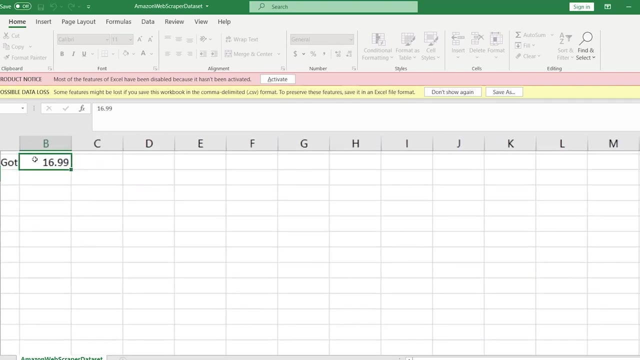 I'm embarrassed. no, I don't want this. okay, perfect, yeah, guys, I, if you can't tell, I'm in need of some. I mean you just, I'm in need of some help here. but I'm just kidding, I'm new, I'm doing fine. I just don't know why that I don't have my 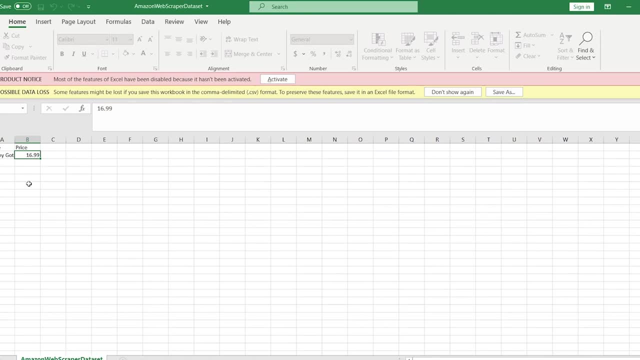 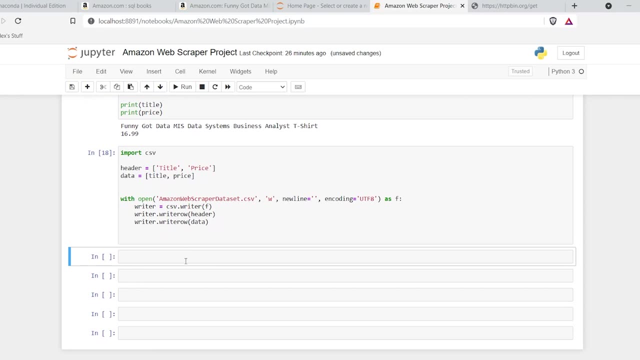 subscription activated. it's not gonna matter for this video, I guess, but that's really random. that's perfect now what we want to do after this, I guess actually what is important is some more useful data. something that I like to do a lot when I do this type of this type of stuff is I like to have some type of date stamp or 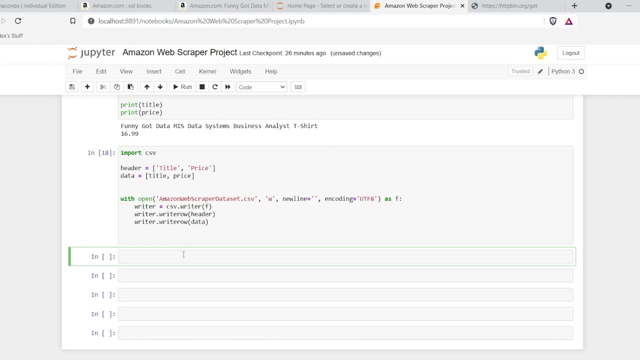 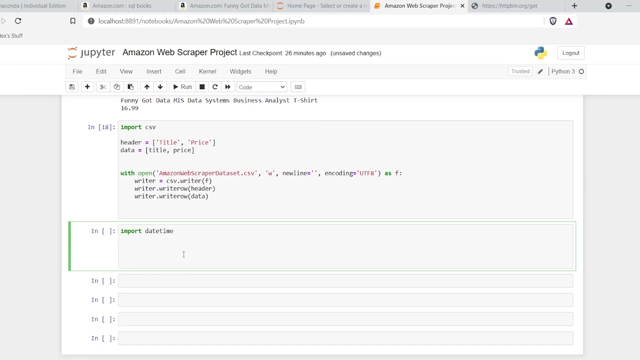 some type of timestamp to know when I collected this data. it usually comes in handy later on. I have never regretted putting it in there. I'll show you really quick how you can do it. you can do import date time. geez, I hate having to format stuff like that and what you can do is you can do date date time and you. 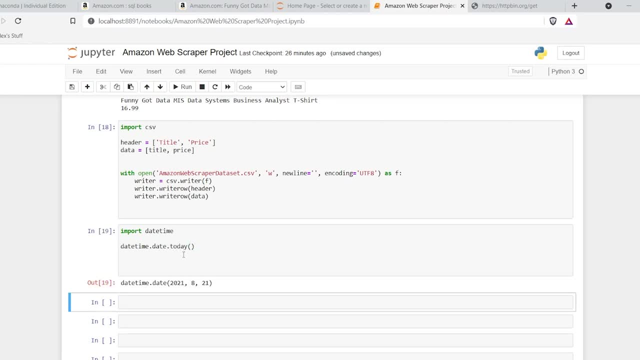 do dot date, dot today, open parentheses, and that is going to give us this right here, and so we're just gonna do: today that's what we'll call. it is equal to this, and we'll say: print today and there we go. so that is today's date is the 21st of August in 2021, so today is. 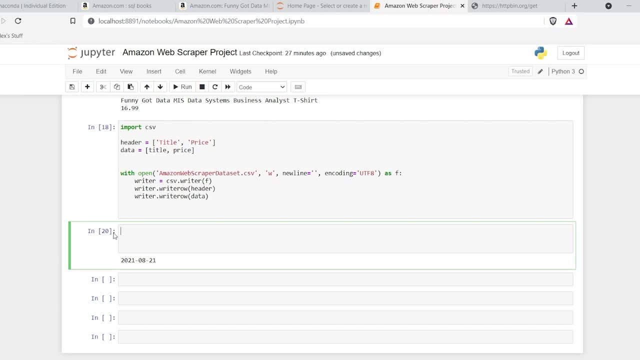 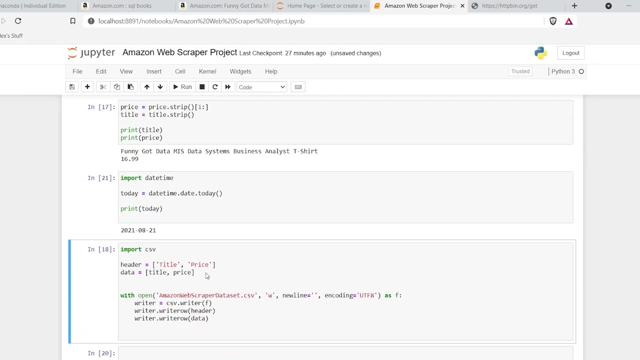 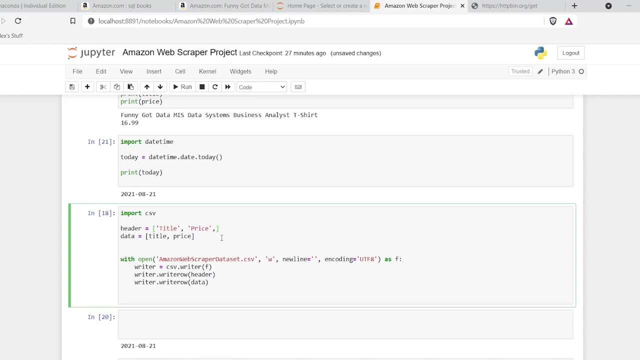 now is now this: so actually I'm gonna get rid of that. I'm gonna put it back up here. I'm going to put it right there. I'm gonna run it again. let's add this right here: we'll do, we'll do, we'll call it date and then we'll add: today. 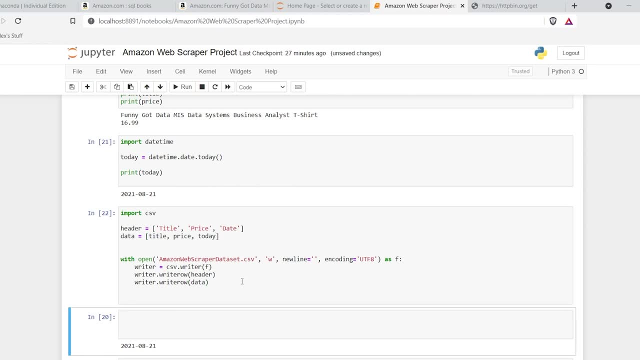 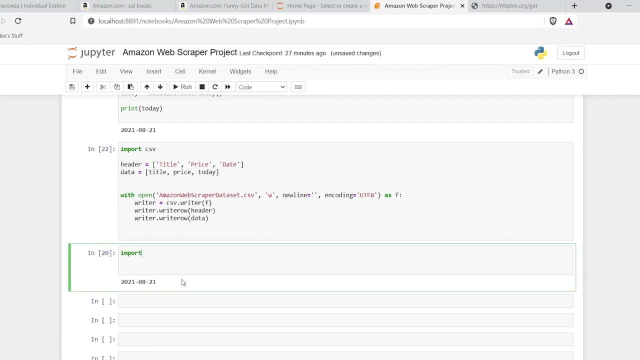 and we'll just run this again, and what we can do just to check the data without having to open up the data every single time, which is super annoying- is running these pandas again. I should have imported this at the top. I'm just kind of I'm not doing this off the top of my head, but I didn't have it 100% planned. 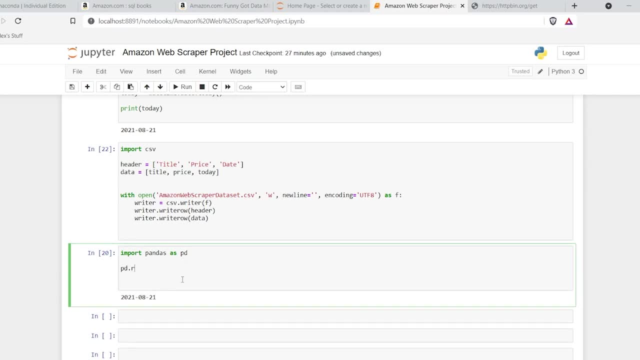 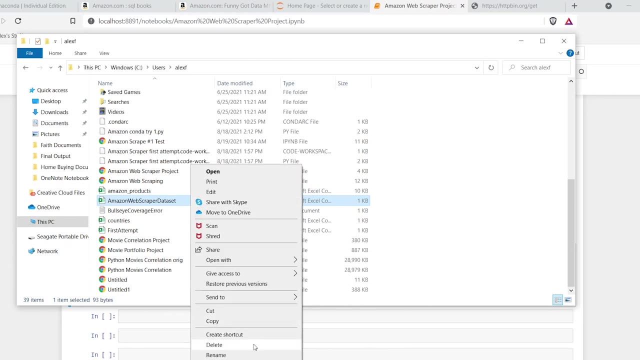 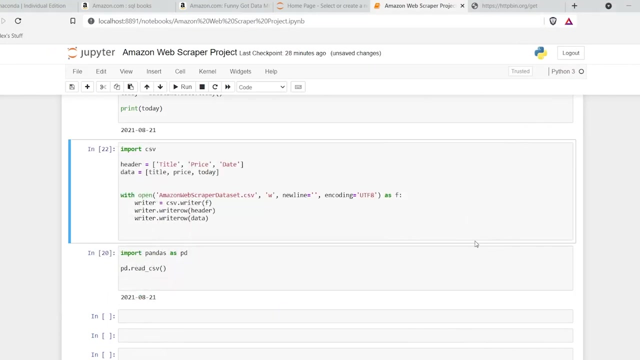 so import pandas and we're just gonna say PD, dot, read underscore CSV and then we'll read it in. what you can do is you can do this by just typing in the data, or what I often do as I go to properties and I go right here: do, do, do. 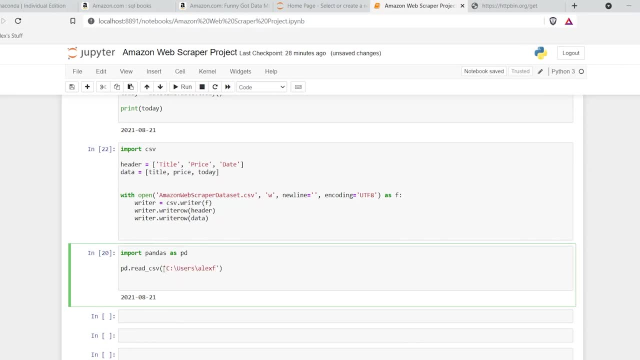 and we'll say: boom, boom, backslash this right here. this I am doing off the top of my head. I don't do this often. I think I have this memorized by now- I, I hope- and then we'll boot print. oh no, we don't have to do print, we'll just do this. what? 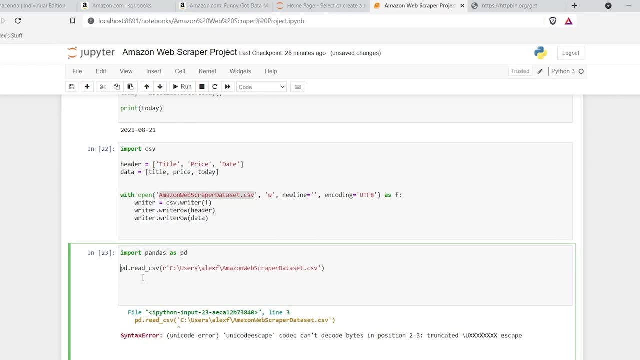 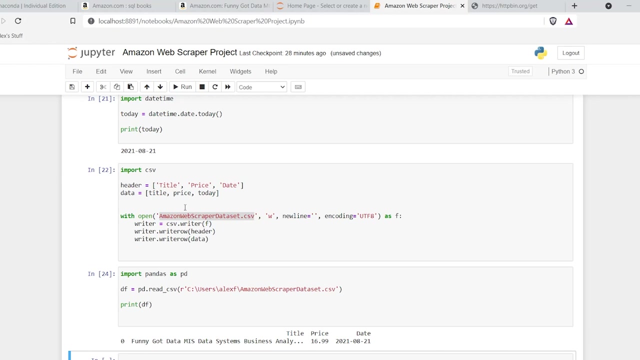 I do are. I'll actually call this data frame and we'll do print. let's see what happens. perfect, okay. so what we have now is the new, our new header, our new data that we added in there. so we have our title, we have our price and we have our date. now 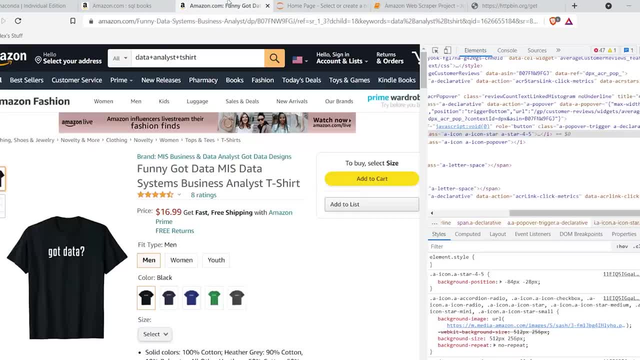 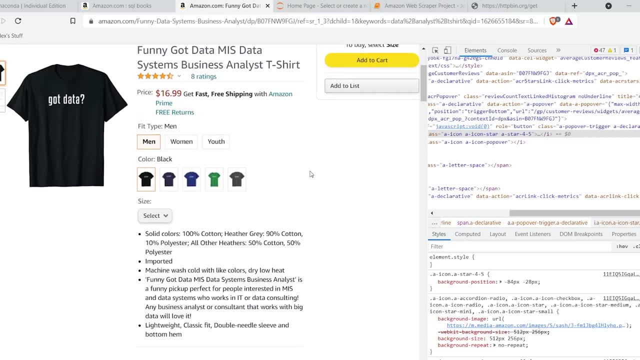 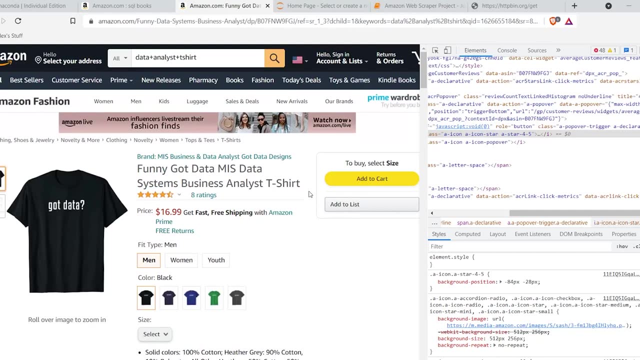 again, you can customize this. whatever you want to add. go back here, you know, find what you want, you know. do you want it to make sure that it has a men's option, or different colors, or you want to pull in this information? whatever you want, it really does not matter, just matters that you know you. 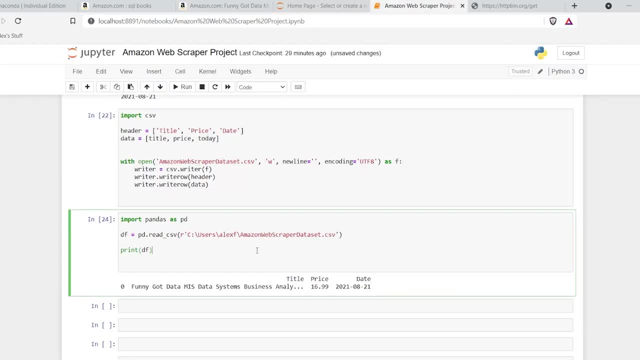 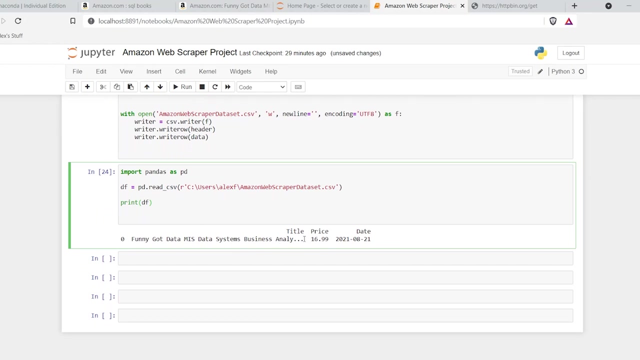 get what you need for whatever purpose. whatever you're making this for, this is more of an introductory video to how to scrape data from Amazon. the next video probably a little bit more difficult and in-depth, but this is kind of let's get you guys started. so we now have this and this is beautiful. 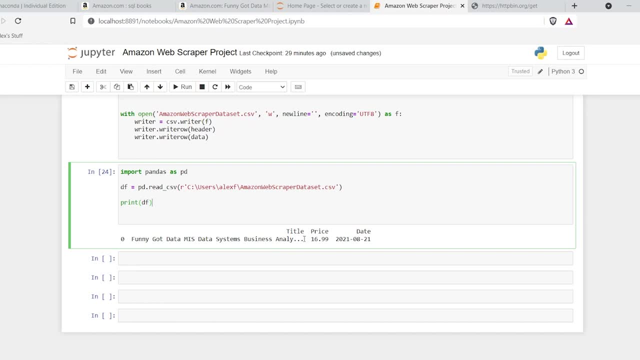 now something that you want to do- when you're scraping data and you're getting, I guess, data over time- and that's kind of what we're doing is gonna be almost like at price tracker over time- is you want to then append data to this so we 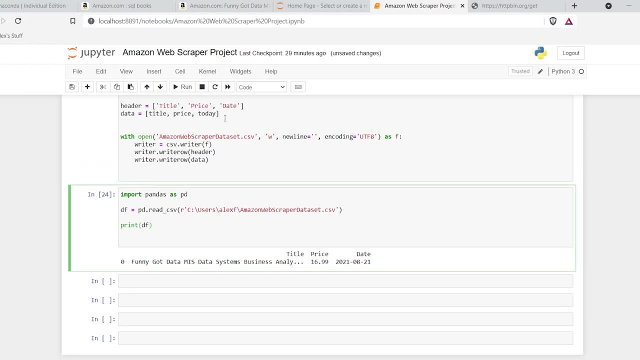 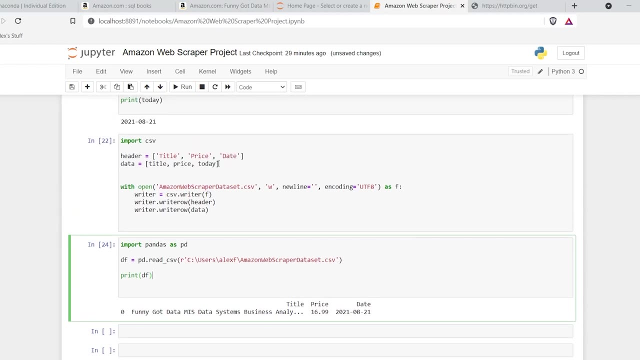 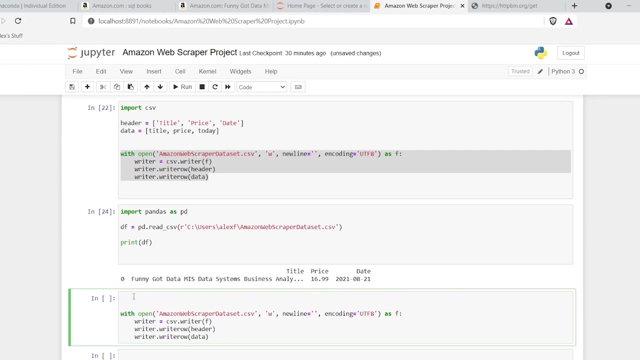 can't only create it, and that's what this does. if I run this a hundred times, it'll only give me this first row. we need to now append data to this. so let's, let's pull this down here again. I'm, I'm not. I haven't added a bunch of notes, I'm. 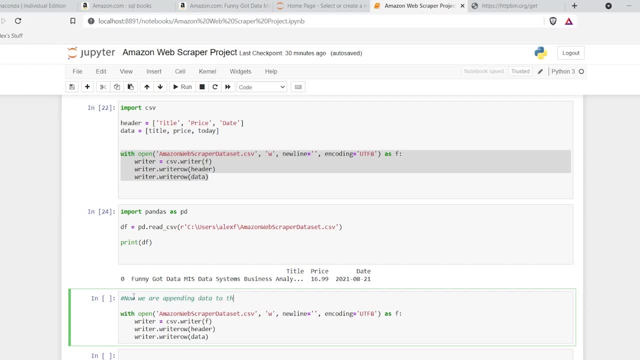 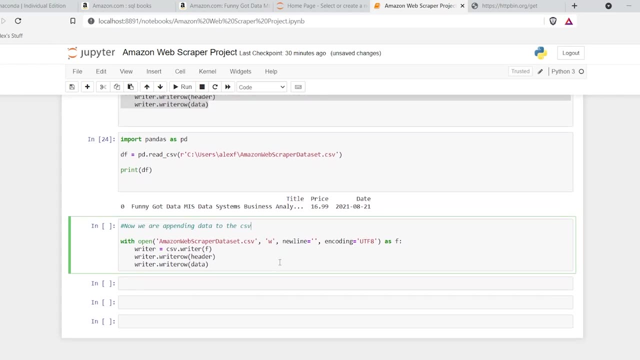 gonna say, now we are appending data to this CSV, I haven't added a ton of notes. I'll try to go back maybe afterwards and add some notes for people who like to read notes. so what we are now going to do is we're gonna change this W to an a. 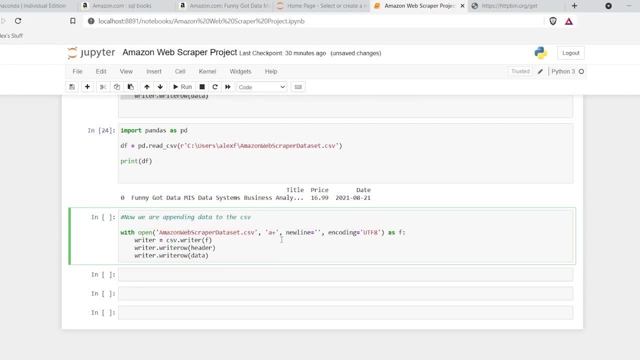 plus. now this is going to be how we append the data and we no longer need to need the header, so we don't aren't gonna do the header anymore, and there we go. so now, instead of excuse me, so now, instead of creating that header again, creating that first row of data again, we are ignoring the data and we're now. 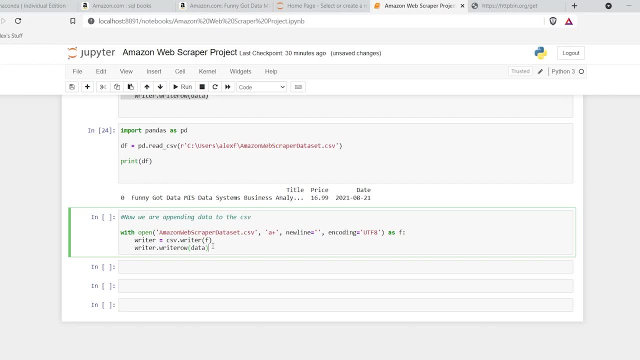 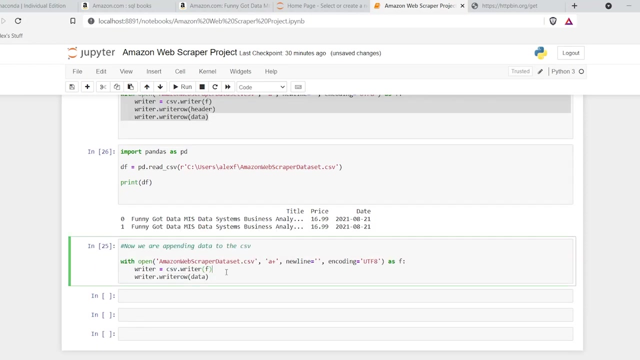 going to the next nearest free row and appending data, which means to add on data to that, and so if I run this- which I'm not going to right now- I mean, why not I can? I can run it and then we can read this in it. so now, there there's our data. I'll run it a few more. 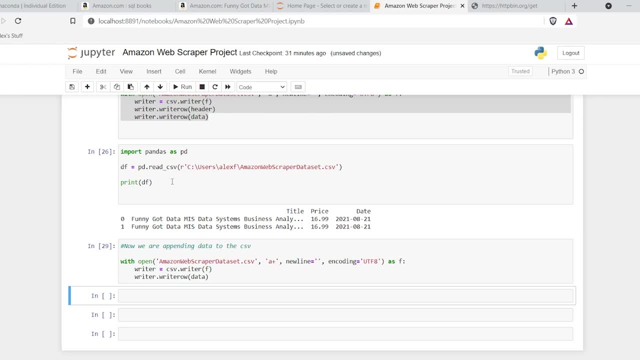 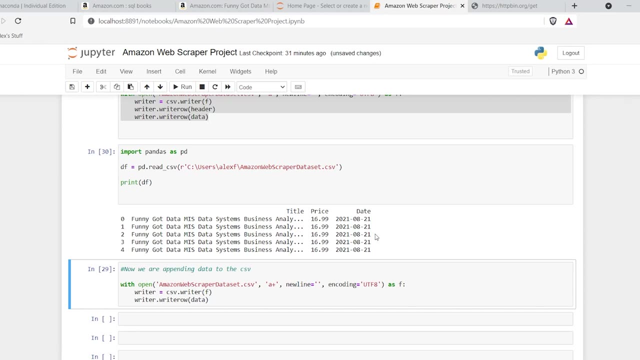 times. I ran it like three or four more times. I run that in and there we go. now it's all the exact same data, super boring, but very, very, you know, good to have now. we don't want to have to come in here and run this every day. let's say: 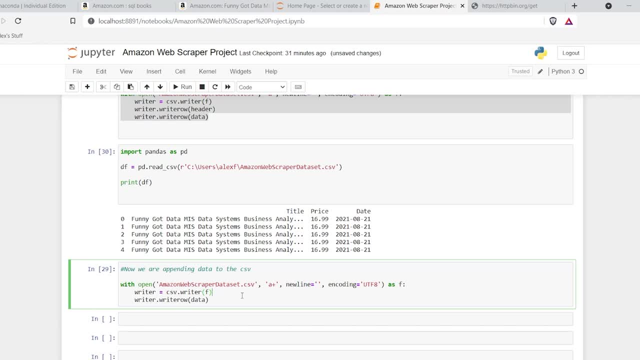 we're gonna do this daily. we don't want to have to come and write, run this every single day, right? we want a way where it does it while we sleep, it does it in the background of our laptop and is easy to do. right? I don't want to come in here. 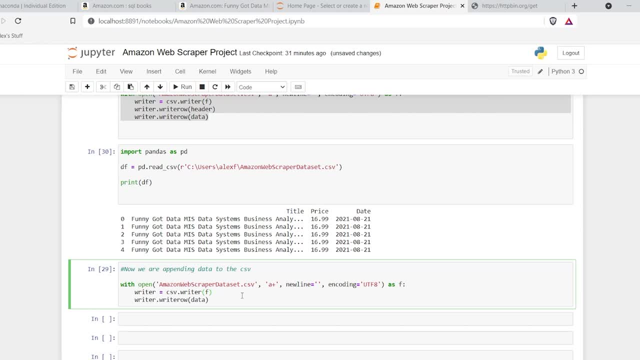 every single morning with an alarm on my phone every single morning. come in here. I want to automate this. so how are we going to do that? give me one second. if you didn't know, I have three kids and one of them is waking up. I'll be right. 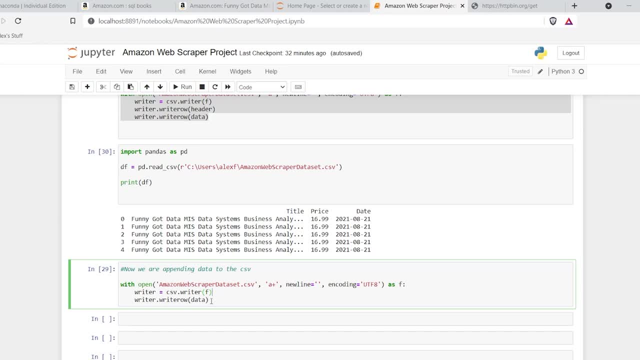 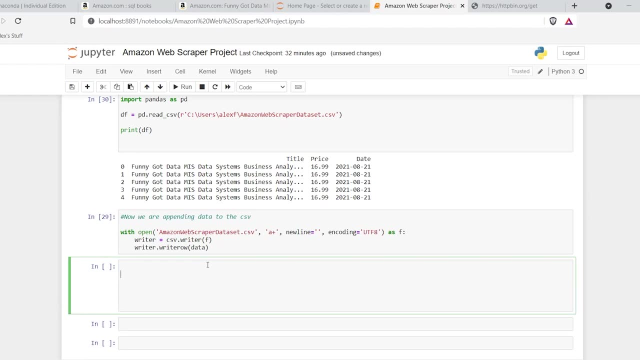 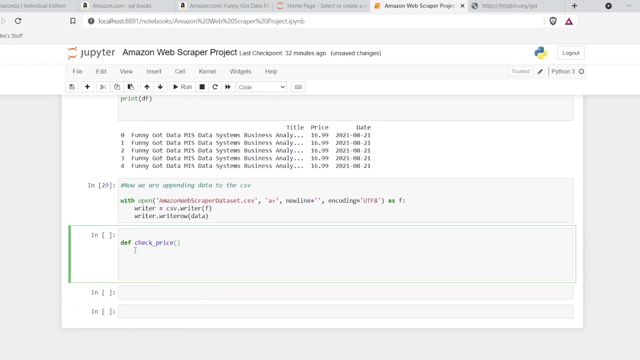 back. all right, I think he is asleep. at least, let's hope he's asleep. so now, what we're going to do is we're going to put this all into this check underscore price. now, you may never have used. oh geez, what are these things called? oh, my gosh, super used all the time. you'll know. 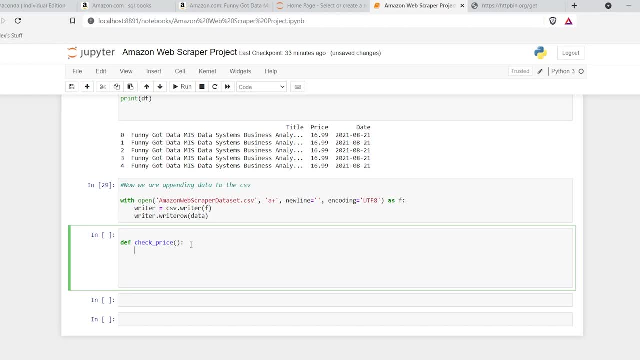 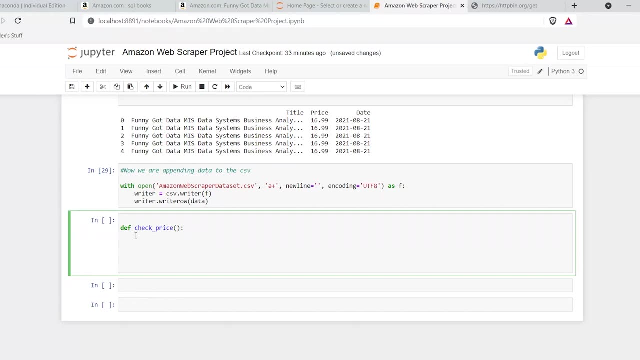 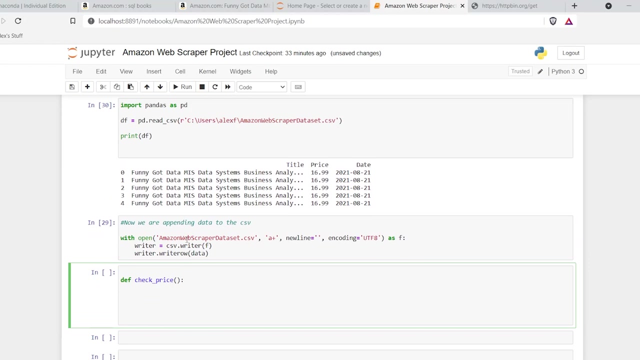 what I what? it is a function, I don't even remember what it's called. maybe there's a function I can't think I'm having, like writer's block or whatever that is. we're gonna put it all in here and then we're gonna be able to use this price check later, because we want to be. 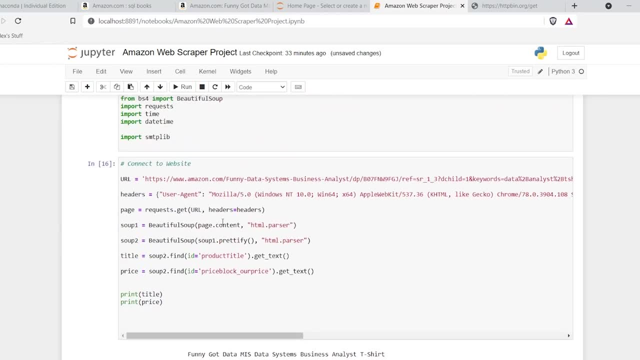 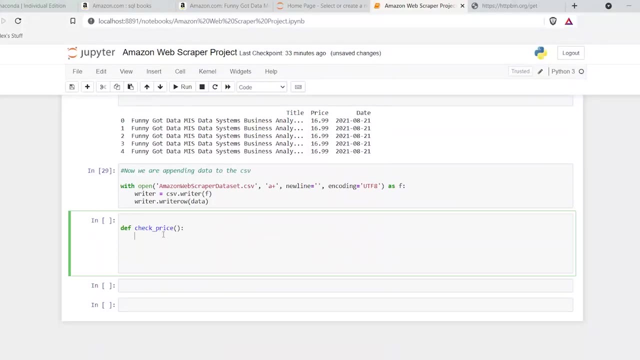 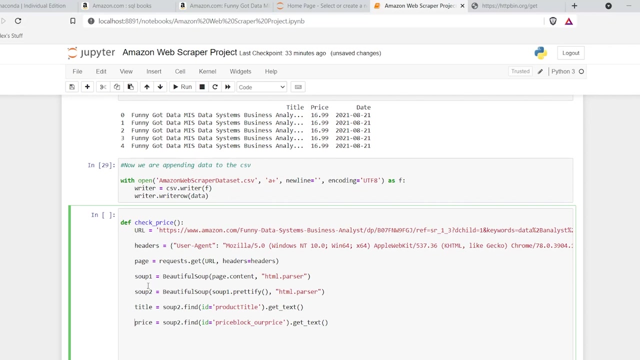 able to automate this. so let's go back all the way up here. we are going to use this, so let's copy all of that in. and oh, geez, all right, everything, just like that. so this pulls in our data, pulls in, or, yeah, pulls in all of our data, all down to the title and the price. 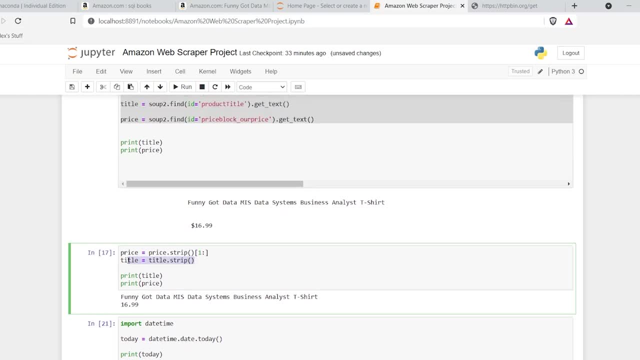 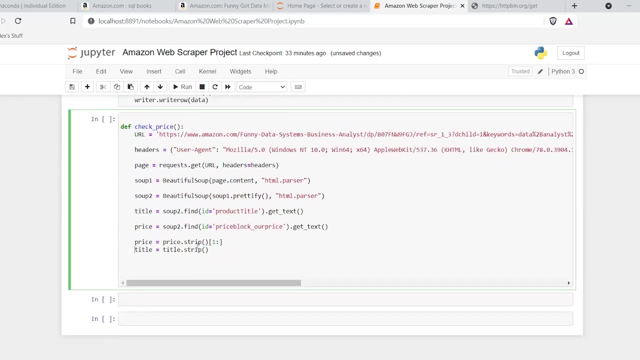 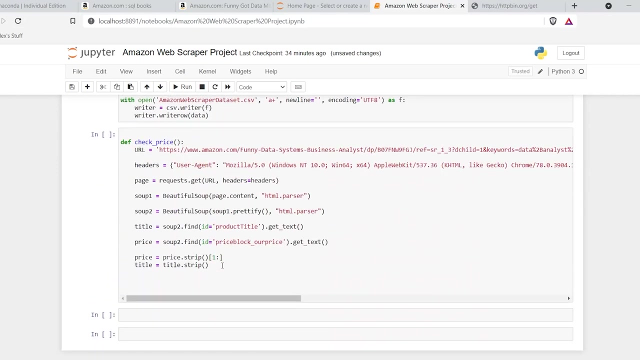 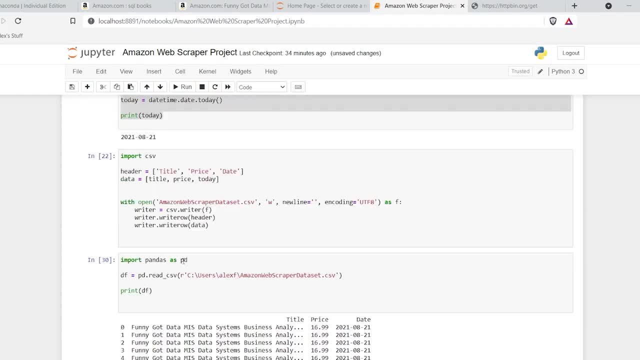 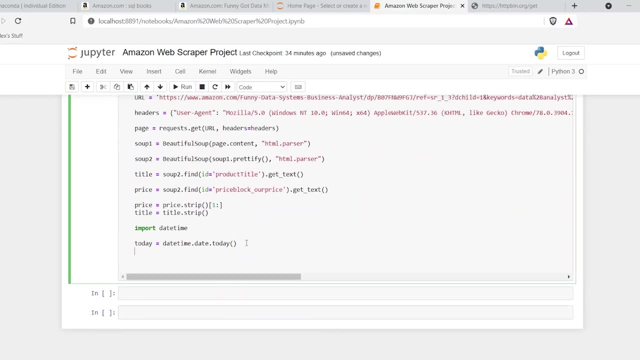 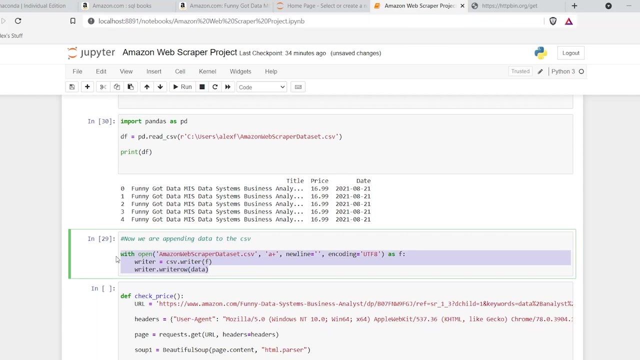 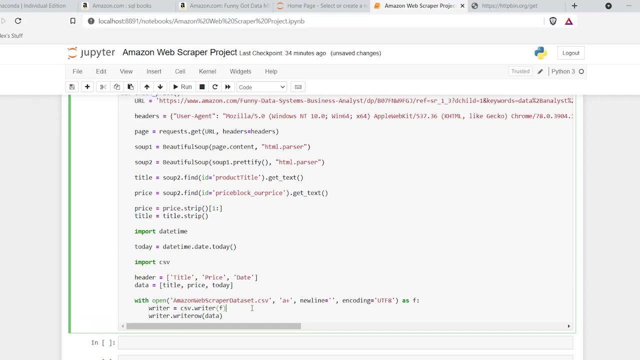 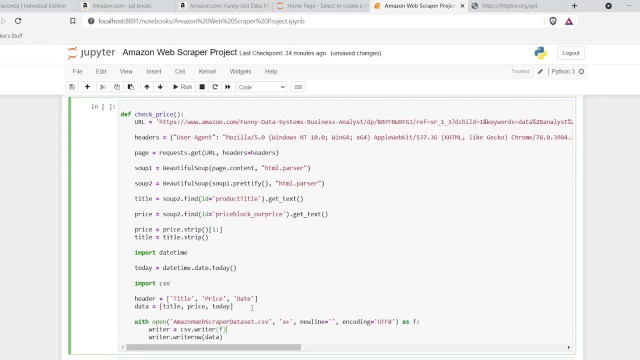 just wrote out. we are now putting into this check price. now you can call it whatever you want, doesn't matter, but let's run that. see if we get any errors. we don't, so this is now good to go. basically, um, what we are going to use this for. um, and what this is going to. 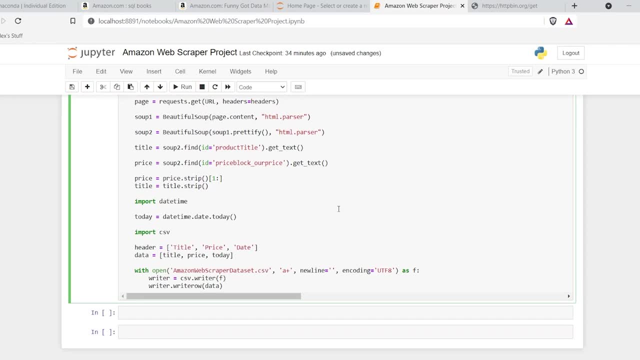 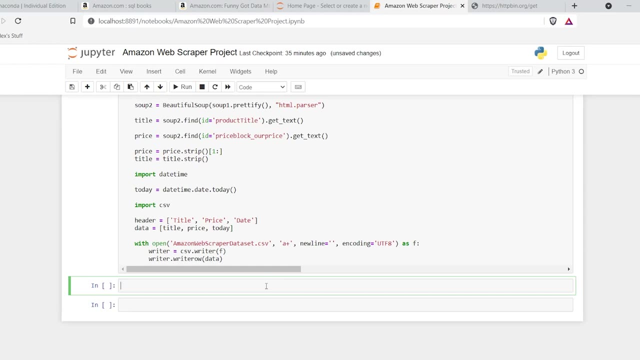 do is we are going to put this on a timer. um, you know, if you ever wanted to like check something once a day, once every 10 seconds, once a minute, whatever you want, and you don't want to have to actually pull up your phone and look at it, this is how we are going to do that. so 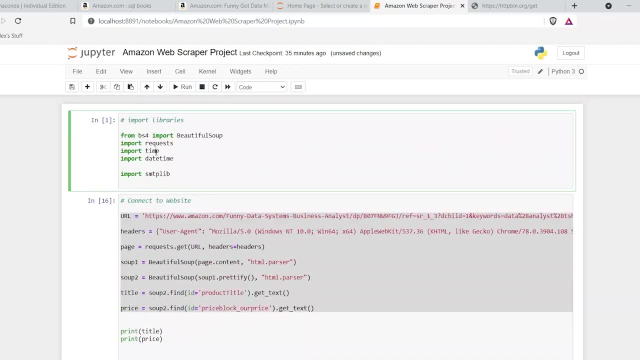 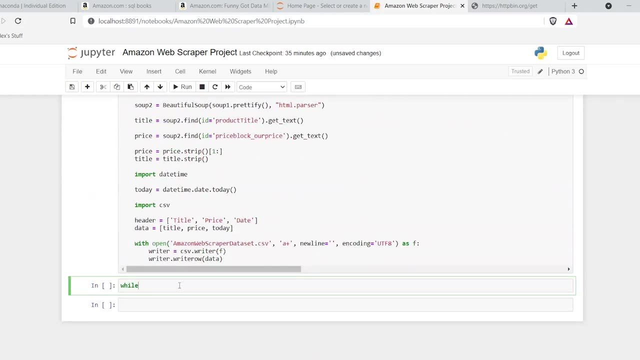 we had something called let's see time, this, this library time, right here. that's what we're going to use right now. so we're going to say while oops, while true, and go like this: do a colon. we're going to say check underscore price. that's what we just wrote out and we do time dot, sleep. 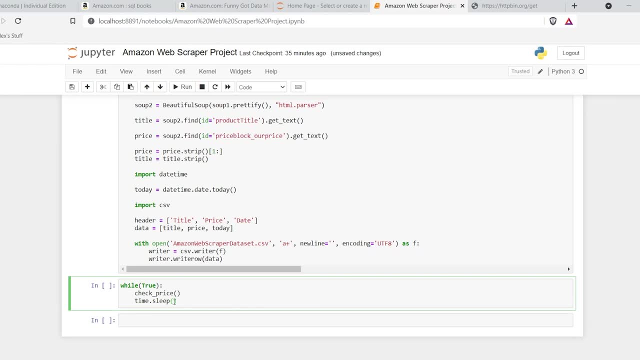 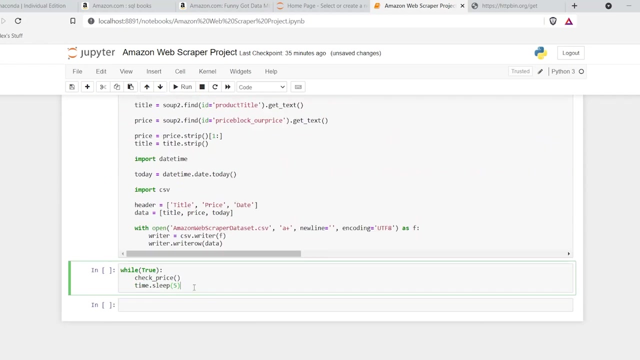 now, this is completely up to you how much time you want to put in here for the purposes of demonstration. I'm going to put five seconds, which means every five seconds. it is going to run through this entire process, and so let's run this really quick, and I'm going to run it for 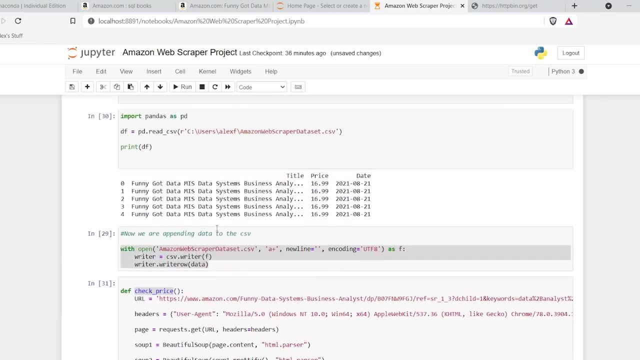 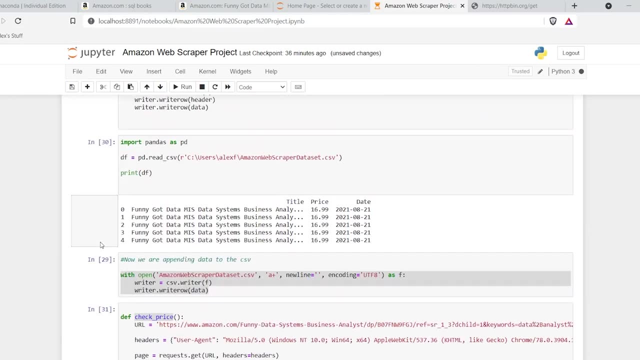 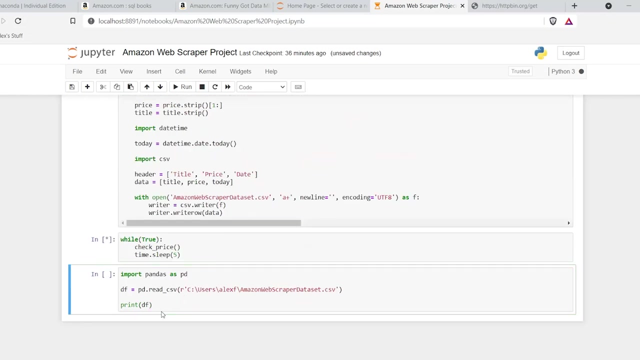 let's say 30 seconds, and then I'm going to pull this in right here. so we just looked at it earlier December. We had four, no five- rows of data, right? What we are going to do is, in just a second, I'm going to stop this, you know. 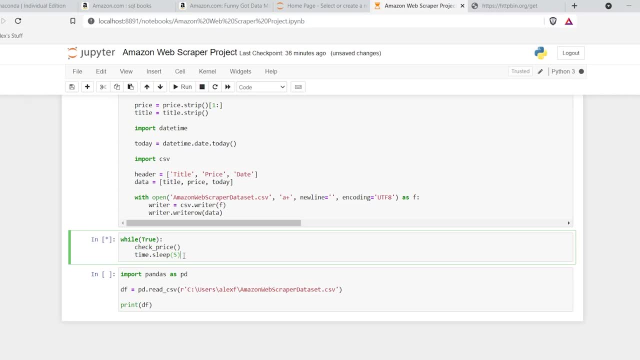 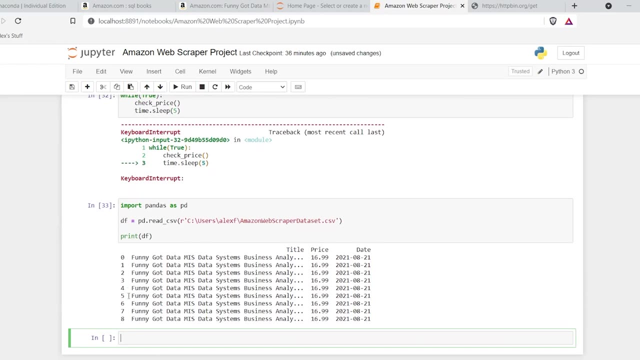 maybe after 30 seconds or so, and we're going to see how much data is in there And let's stop it right now. It's been going far enough And now let's run it. So now we have five, six, seven, eight. 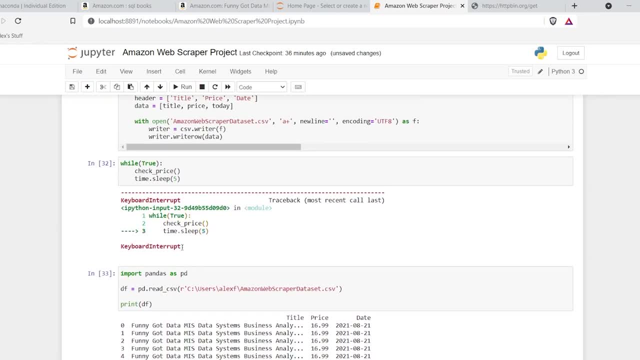 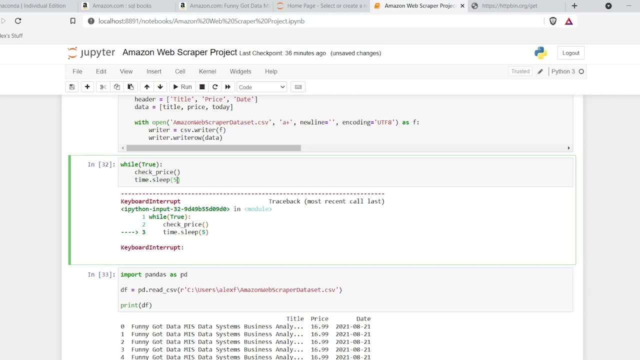 So I guess I ran for 20 seconds. We can. that was for demonstration purposes. I've never do anything every five seconds, unless it was like Black Friday on Amazon. We can put this as long or as short as you want. You can run it every second if you want. 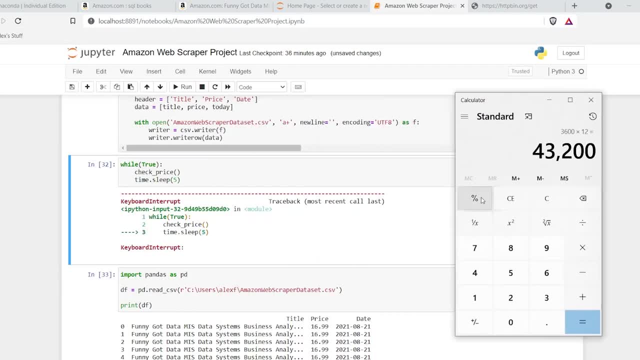 That doesn't make sense to me, but you can. What we can do is do a little bit of math, And I don't know this off the top of my head, So I'm going to do the math with you. live, Pretty exciting stuff. 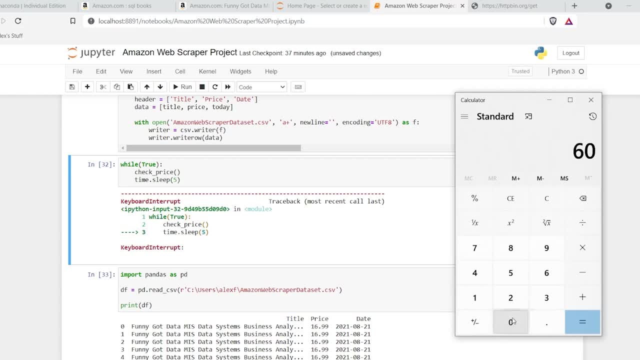 Got the calculator out. So there are 60 seconds in a minute And this goes by second, By the way, and you could do- you know you can do- some string up here of calculating this, but I'm just going to put in the number because it's easier. 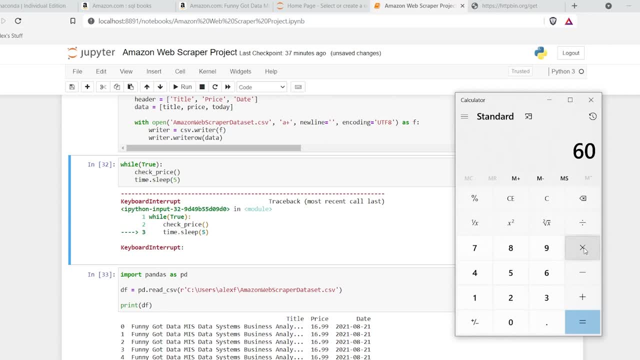 Maybe not easier. I'm just going to do it. There's 60 seconds in a minute. There are 60 seconds or 60 minutes in an hour, So that's one hour And we can do 24 hours in a day. 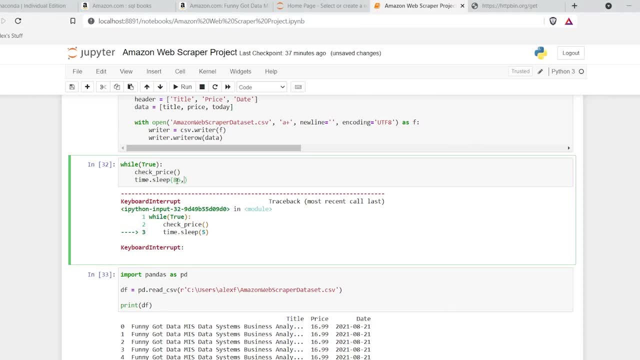 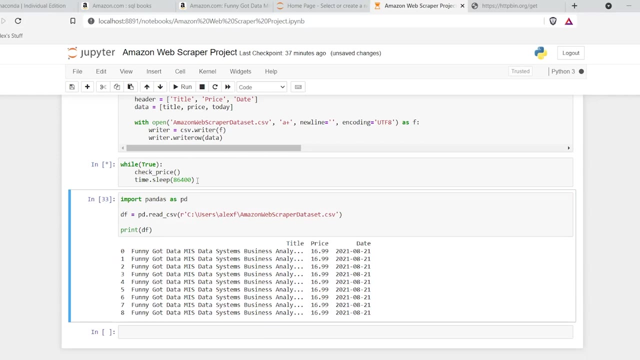 So that's 86,000. I believe. Did I read that right? Oops, Did I read that right? Yes, So this: now, if I ran this- and I'm going to this- is going to check the price every single day. 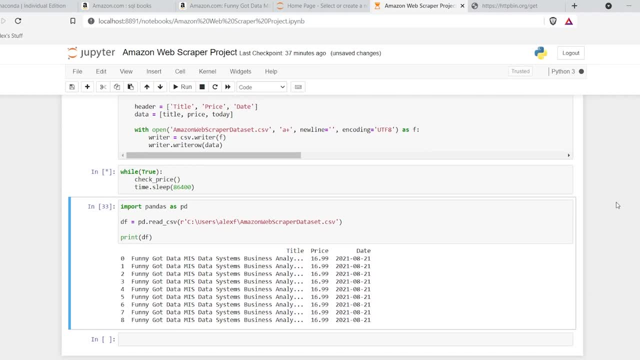 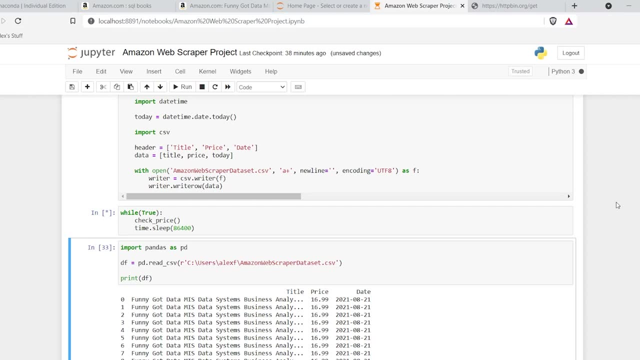 And this is the entire point of this project- Not the entire point, but this is a big part of this project- is we want to create our own data set. Now, something that I personally really love is a data set That has you know that I can do some type of time series with. 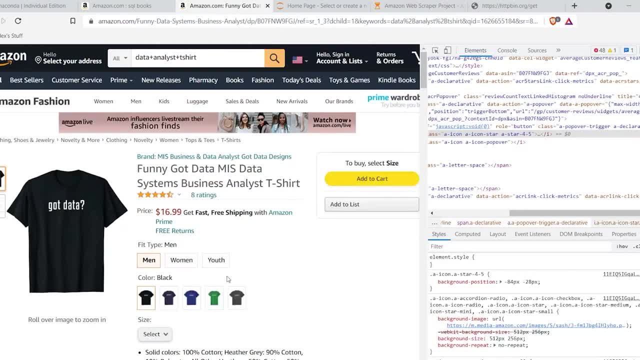 Now this is not exciting. It's probably not super exciting for this right, But you get the idea that if this price were to change, we would then see that reflected in the data at some point. You can do this on any item you could ever imagine on Amazon. 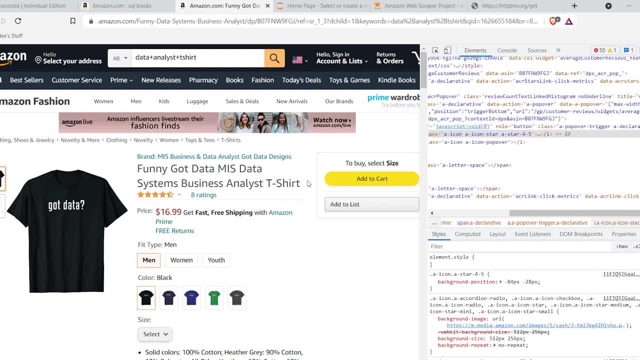 It's the exact same process And some items change often. This t-shirt, It will most likely never change, And so you know again. this is for demonstration purposes. The code itself will be nice to put in a project, although the data set. 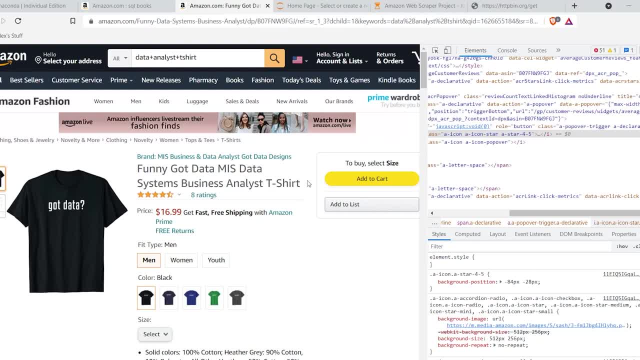 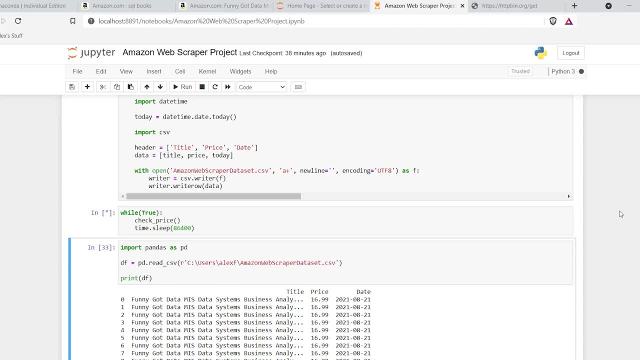 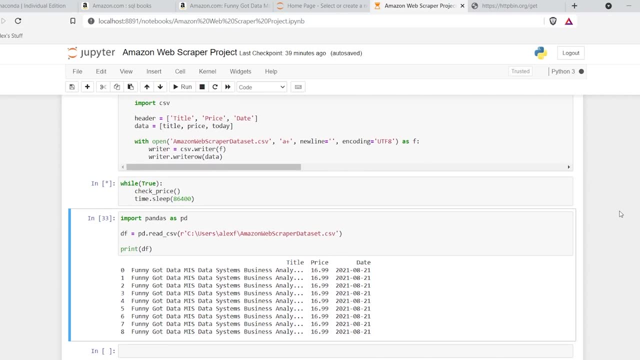 that you get from this probably won't be the best I would imagine, but notice that this is running. I can then minimize this and this can run on my computer, basically as long as my computer is working. One thing I will say before I go on. 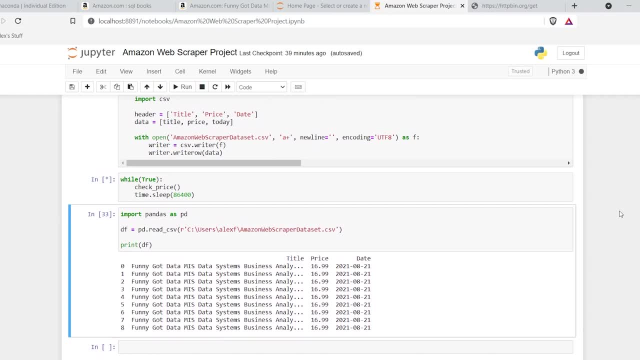 Yeah, Some more stuff. One thing that I will say is that I, personally, when I did this for a, when I, um created this, I did something similar and I put this in visual studio code, Um, and I didn't put it in Jupyter notebooks. 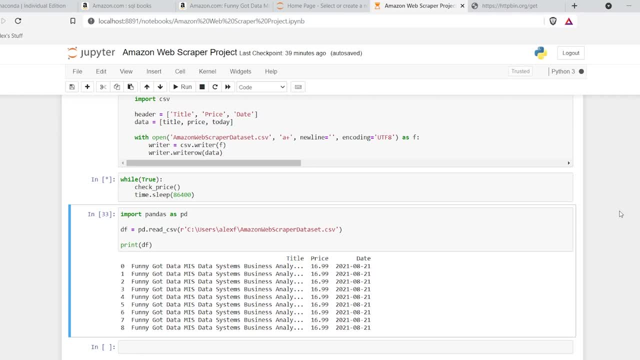 That's a personal preference. I would look into that if that is something that you want. Um, I think visual studio code is a little bit easier for automating these types of tasks. Um, but for illustrative purposes And for demonstration purposes, you cannot beat Jupyter notebooks. 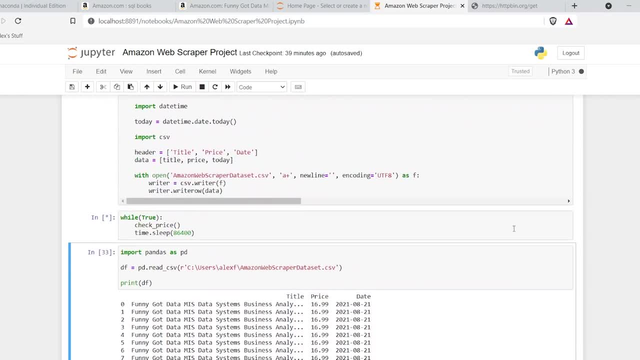 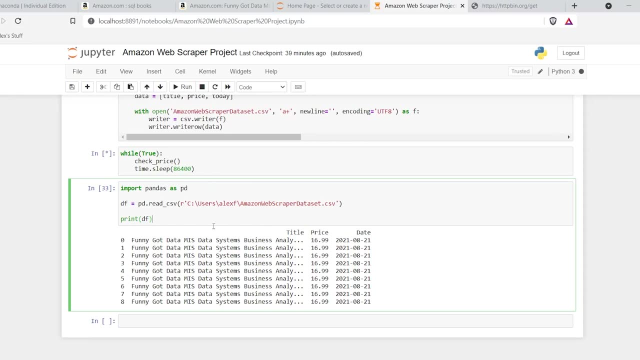 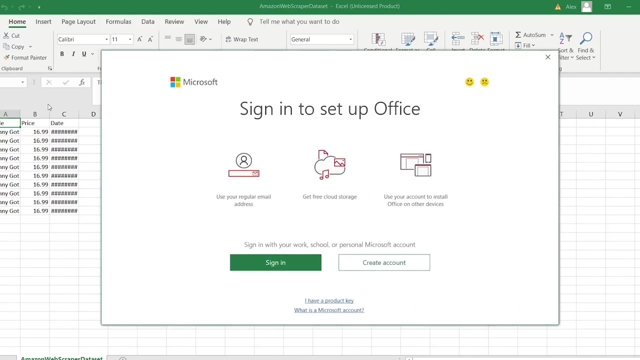 That's why I did it. So, with all that being said, that is basically the end of the project. Now, um, I'm not going to stop this and read it again, but you get the point. Um, we now have, um, a data set that- oh geez, all this again- that now has um. 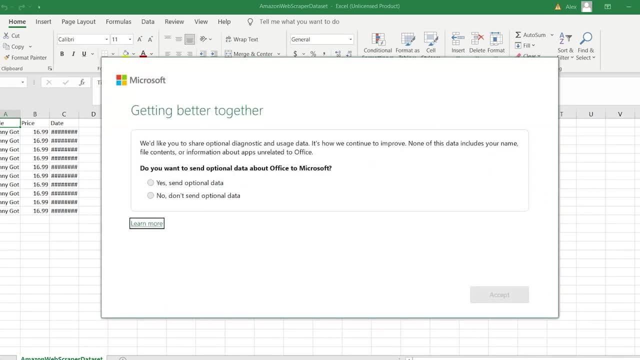 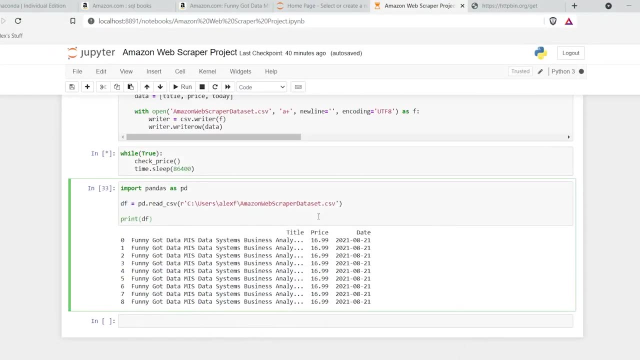 data. I'm getting out of here. Oh geez, it's hounding me. Let me get out of here. Oh no, All right, This is embarrassing, guys, I'm embarrassed. We now have a CSV file with data in it. 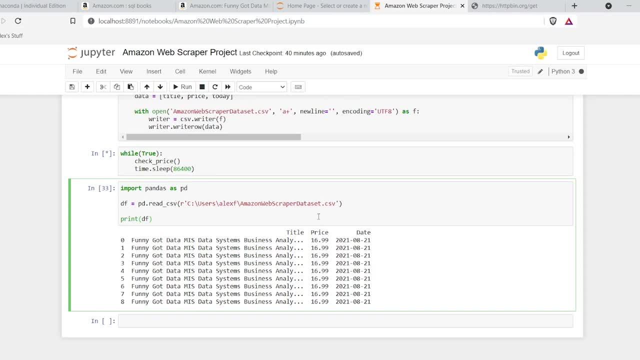 Now you run this in the background of your computer. You can do that. I have done it. I've ran it for weeks. I have ran it for months. Um, if you restart your computer, just come back in here and restart running this process. 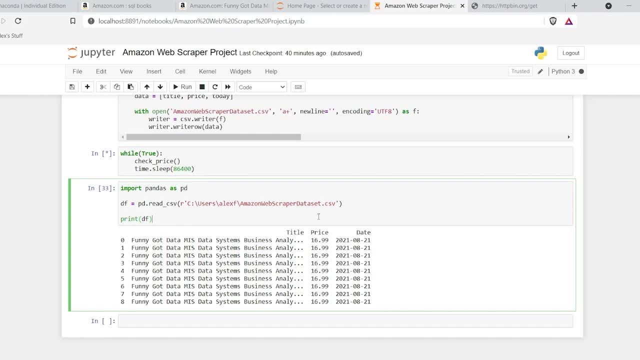 Um. it's the same for any automated process, unless you start using some online um automation service which will run it regardless of your computer. They do it, you know, either in the cloud or on- Okay, On some um server. 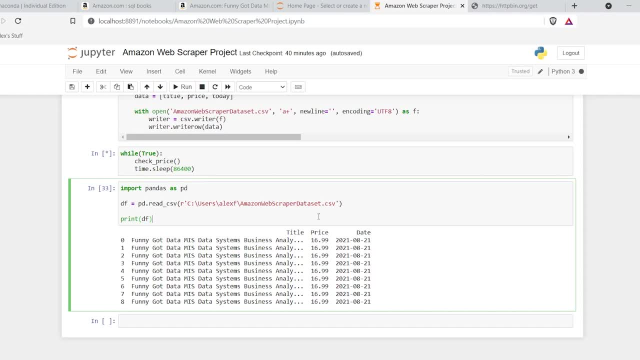 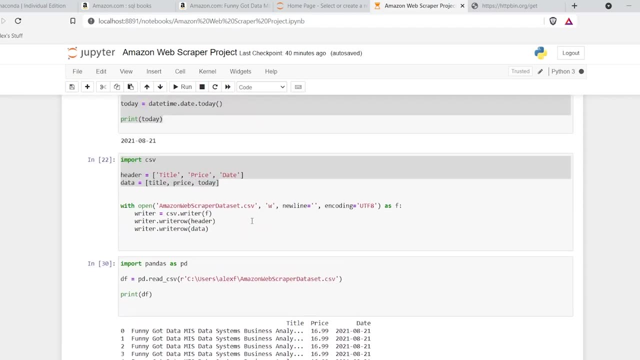 So you know that this is a really good option. Again, if, if you restart your computer or something happens, you lose connection, just come in here, run this through the script again. um, except for the one where it deletes all your data. don't run that one again, only run that one time. 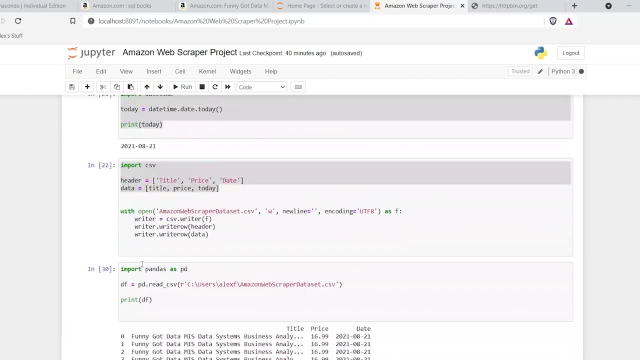 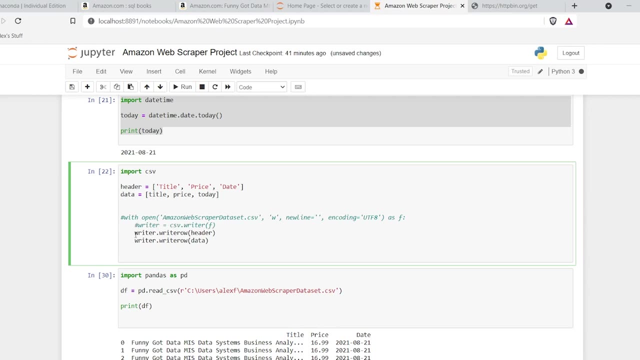 Um, and then you will, And in fact, what I would do is then: um, I would just comment this out, right, I'd come in here and I would just comment this out, So that anytime I come back in here, I would never accidentally delete all my data. but 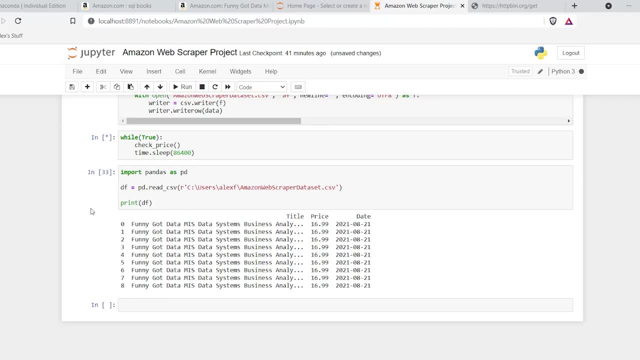 that is what this project does now: something really interesting, something that I have done in the past that I thought was really cool, really useful. I actually did it for um. I actually did it for some watches that I was watching especially. 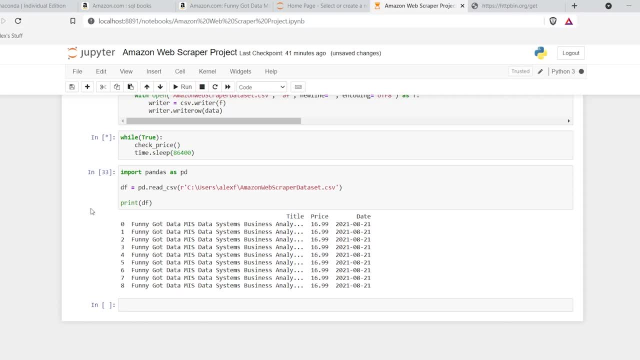 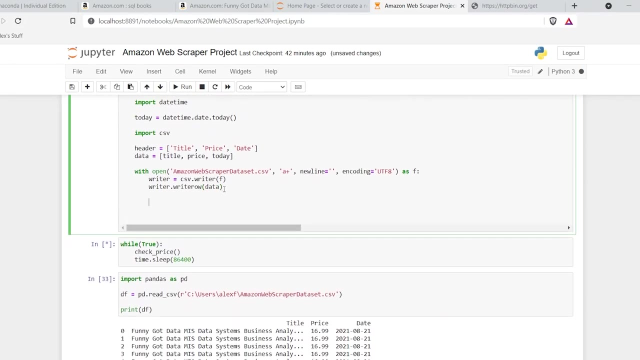 on black Friday- It's when I used it- I was interested in a price drop or price specific price chain, And what I did was, as I said, and I don't know. so what I basically did was is I said: 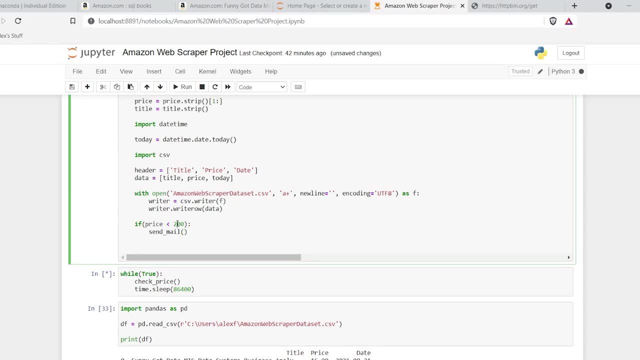 if the price is lower than, let's say- let's say, we want it to drop below $14,. it would then send an email. Um, and I'm going to show you the script that I used. It still works, Um, and if this is something that you are interested in, I'm going to show you the script that I used. 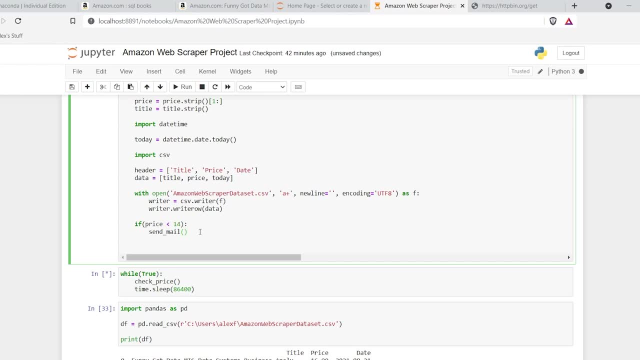 Um, and if this is something that you are interested in, I'm going to show you the script that I used, And this could be a completely different project. I just think it's interesting And I wanted to show it to you, Although I wouldn't say this. this is part of the final project. 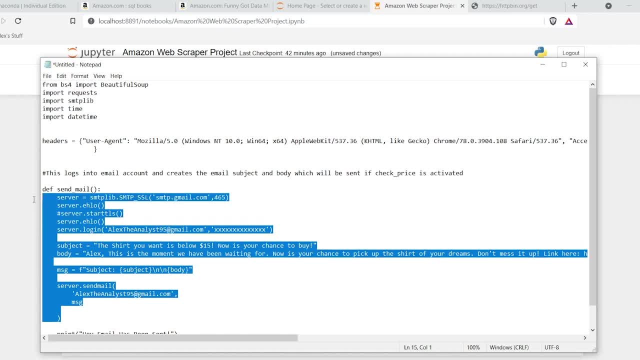 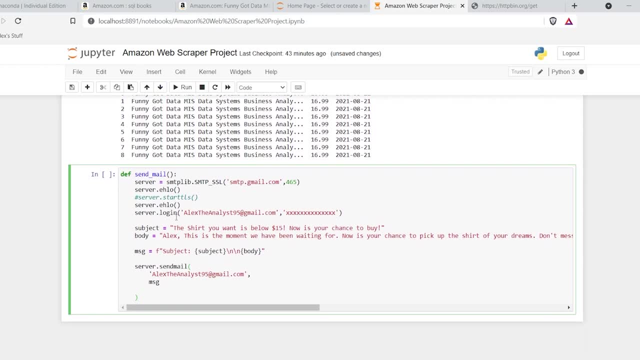 Let me just come in here and we're going to create this super simple- Um, not super simple. We're sending a mail, We're connecting to a server. We were using Gmail. We're logging into our account. That is my email. 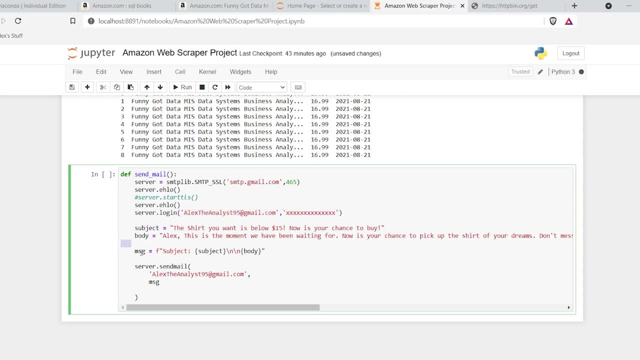 You will not get my password. We're getting the subject, the buyer, The body, um, we, we configure or or just kind of create this message and then we send a mail. So then I have this: define uh, or this send mail. 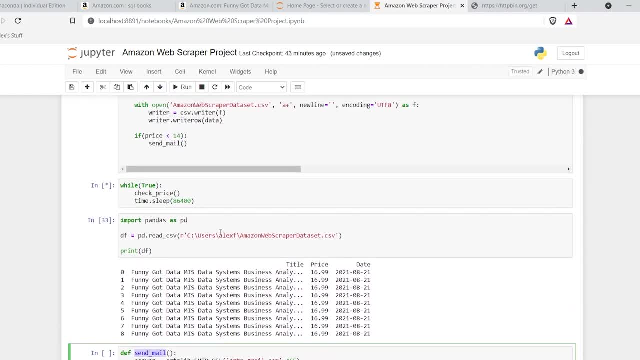 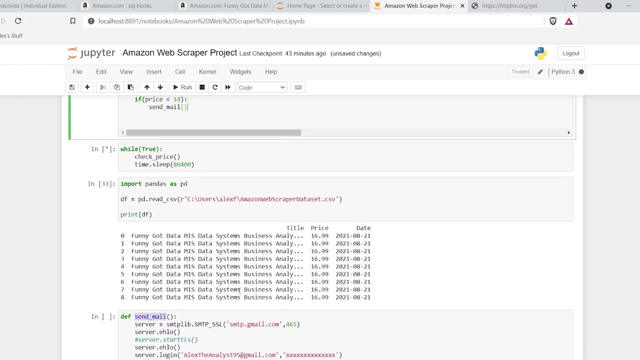 I. I am blanking on what this is called. I'm going to call it a function, but that's probably not right. So if that price drops below a certain point, it'll send me an email. Um, I have used this, and I used it and was able to buy a watch that was, like you know, let's say, 140 bucks for like 90 bucks. 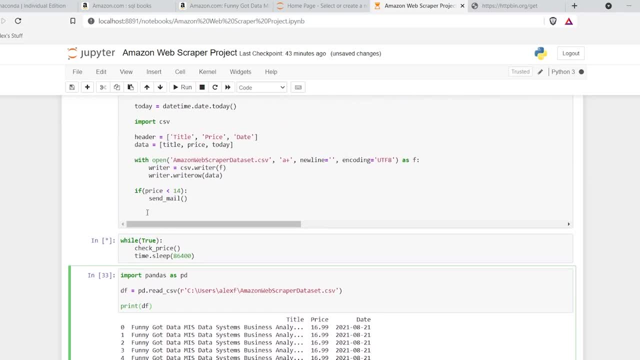 I'm on a black Friday sale And I was really, really happy about that, So this can be used in that way as well. Um, not something you have to write into your project, just something I'm going to include down here. 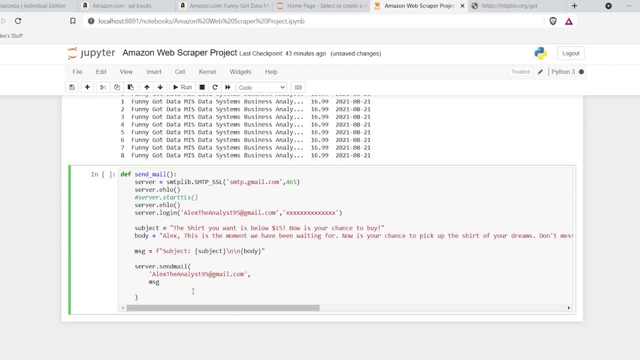 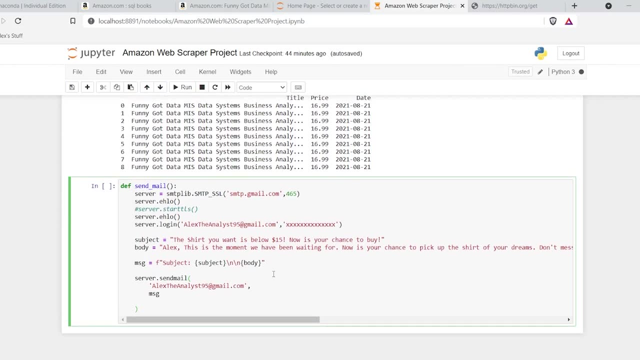 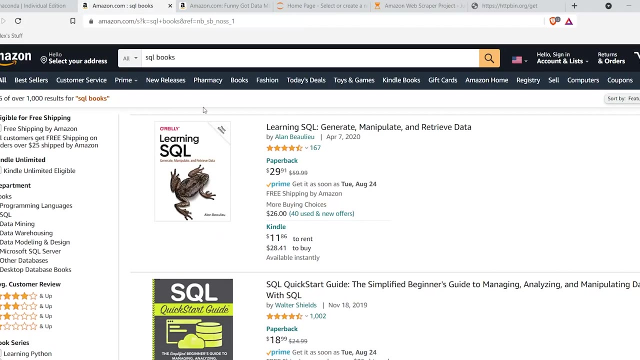 If you want to try it. I think it's super interesting, Something really fun, Um, really fun to mess around with. I enjoyed this. So, with that being said, uh, this is, this is the project Um I in the next one, and I promise you, this one is probably going to get a lot more. 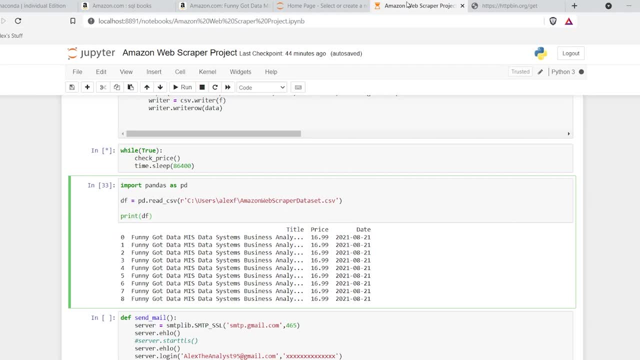 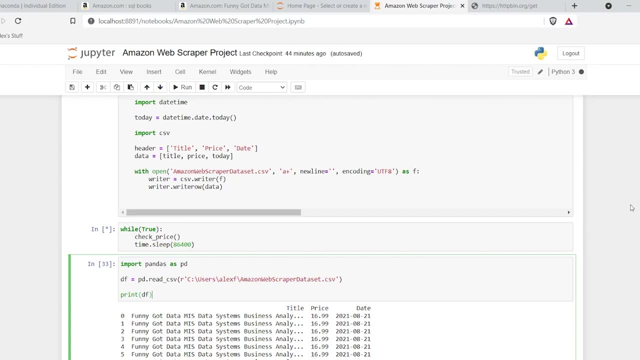 Difficult. if you thought this one was easy, which I hope, maybe I hope you do- then that means you're pretty good at Python. you know, in the next, the next um web scraping project, And I hope to do many of these. 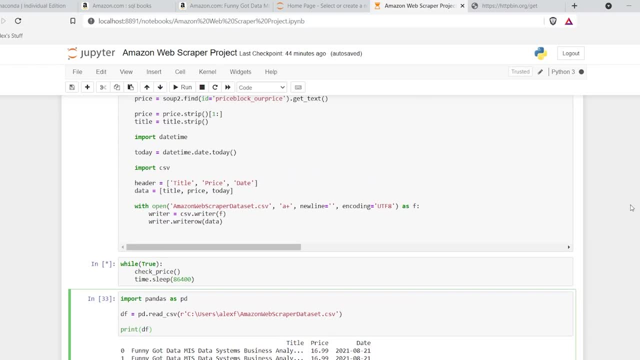 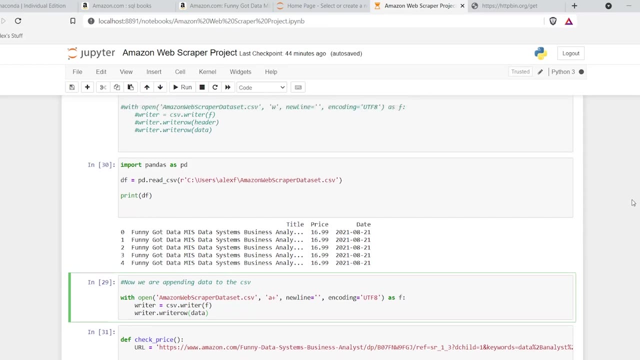 I might do um, even all the ones that I put in that poll, but I started with the one that was the most popular Um. you know, if you were able to get through this, I think that that is fantastic. I think this is a solid project to create um a dataset. 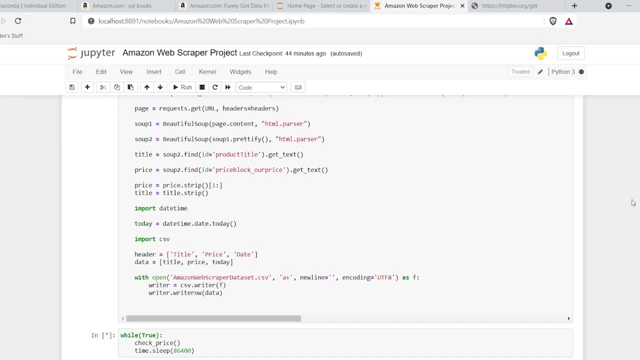 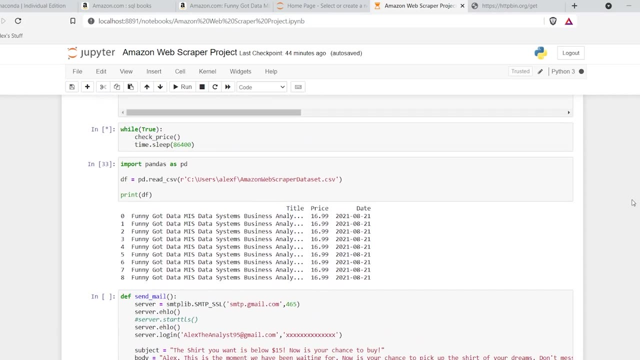 And so use this how you will. you can copy my code Exactly. I don't have a problem with that. again, I don't think this is beginner. There are some a little bit more um advanced things and I know I know in advance, just like intermediate level things um that you kind of learn as you get into it. 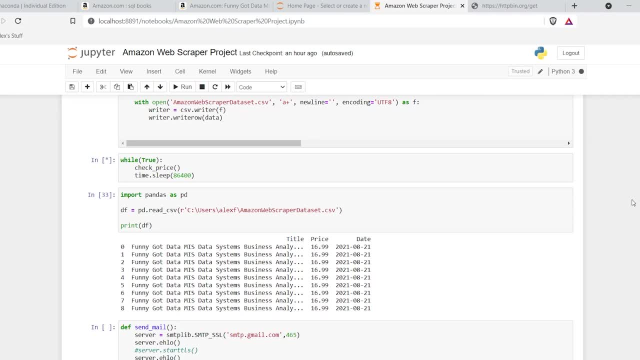 And so, um, I hope that this was instructional. I hope that I explained it. you know well, um, and I hope that this is useful again. you know, when you actually use this, you'll have 22,, 23,, 24.. 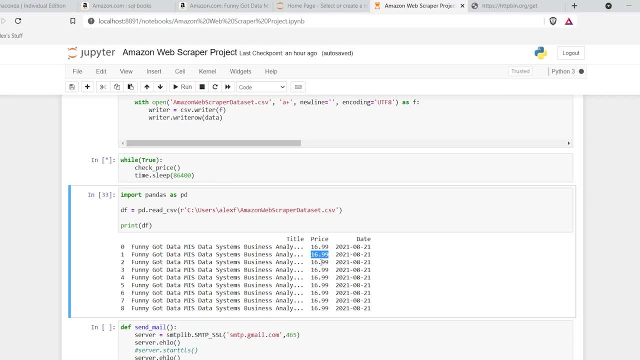 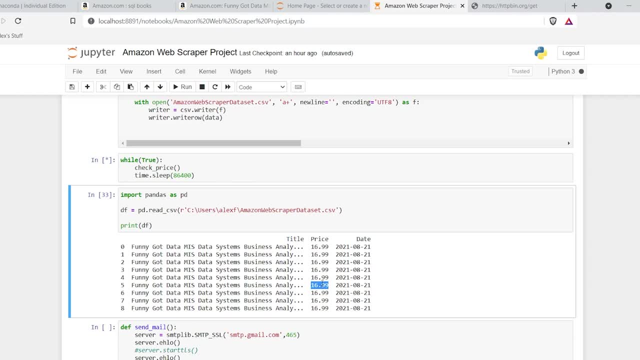 I promise There are some that literally change almost every other day, like down a dollar, upper dollar, Um, and then black Friday just goes crazy, um, with these price changes. So use this as you will. I hope that this was instructional. 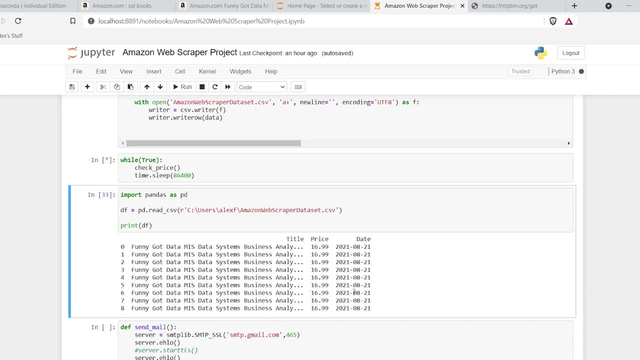 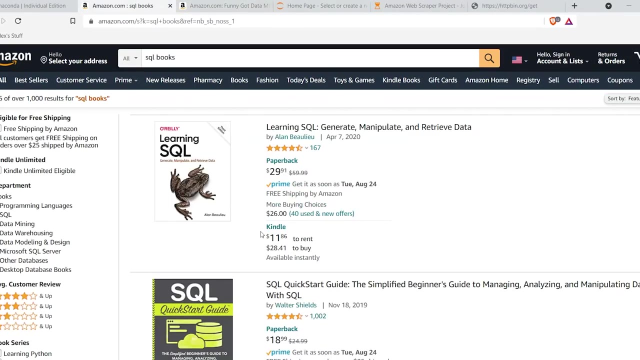 I hope that it's Useful. Um, I think I said that before is I, you know I I'm doing this because I think it's really interesting, It's really useful. Um, this to me again was a good introduction, a really good introduction to web scraping, because in this next one it gets quite a bit more difficult. 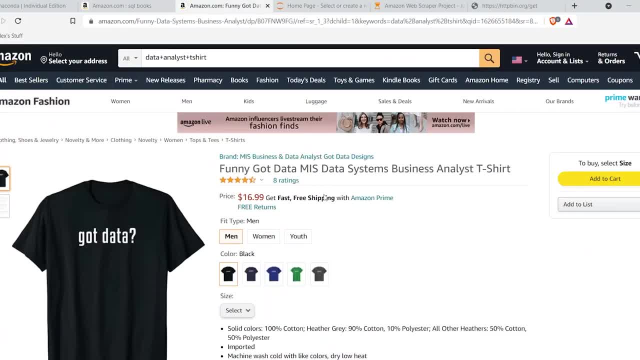 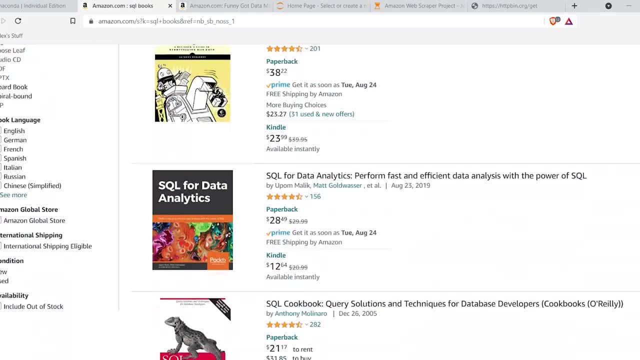 Um, I would say, on a scale of like difficulty, this is like maybe a four and it'll probably jump up to like a seven on this next one. Um, just just much more Um, technical or or coding heavy. So, um, you know, look forward to that. 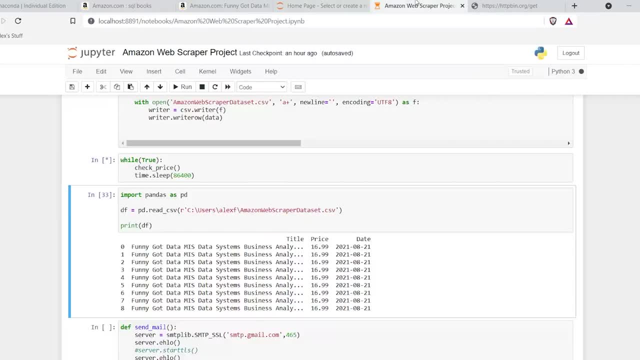 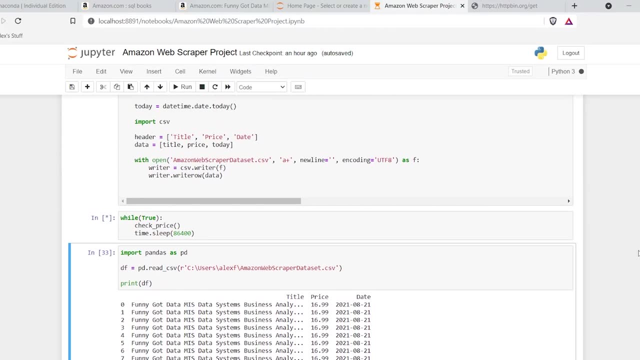 If that's something that you look forward to. with that being said, I'm going to go back over here for my send off. with that being said, I hope this was helpful. I hope that you learned something. Um, don't get mad at me if it was too easy.